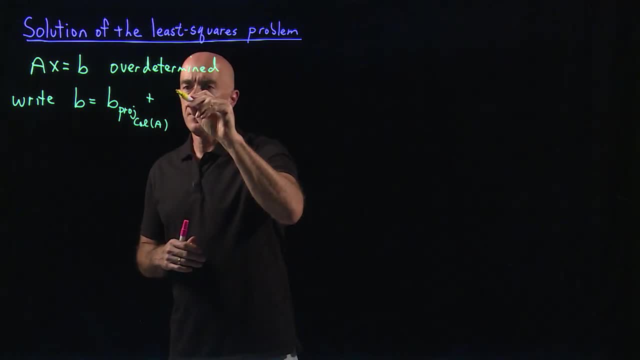 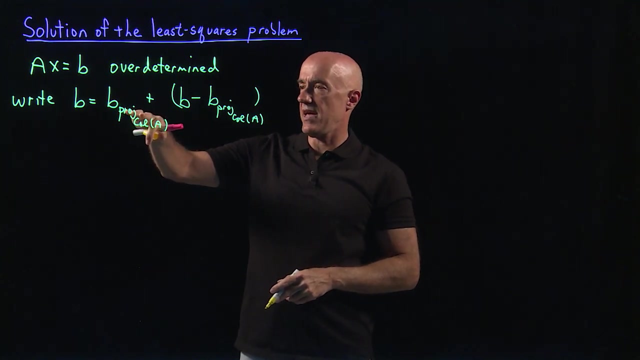 or orthogonal to the column space of A, which we can simply write as B minus B projected onto the column space of A. So B is split into two pieces, So B is projected onto the column space of A plus whatever is left over, So whatever. 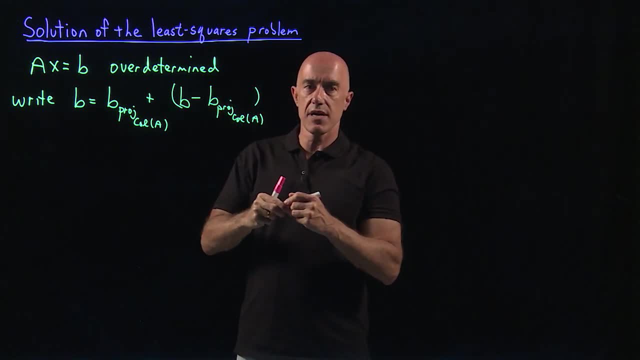 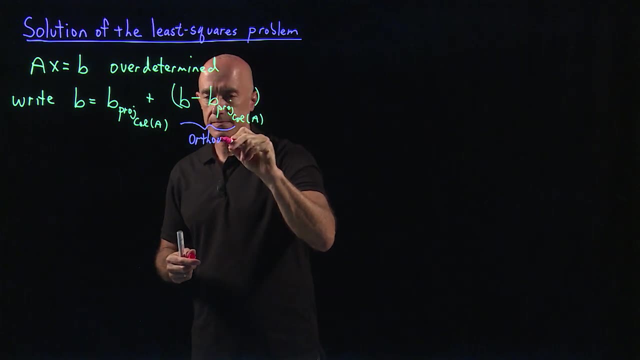 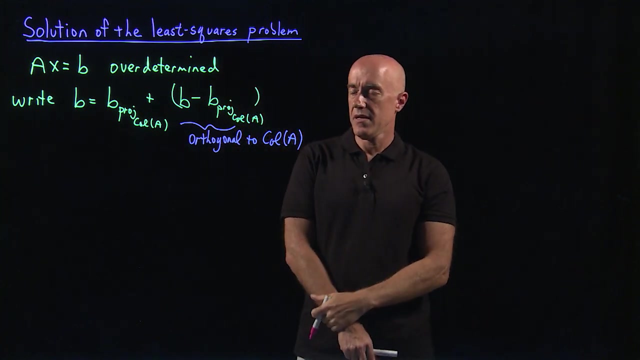 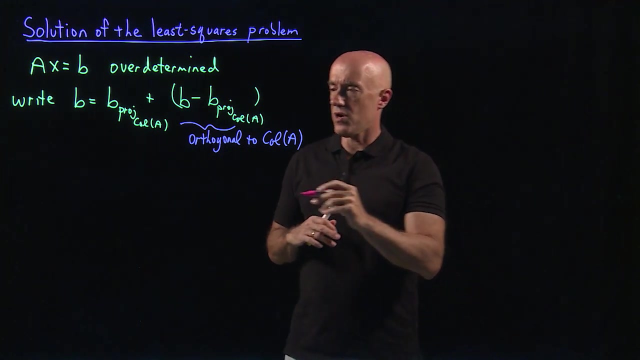 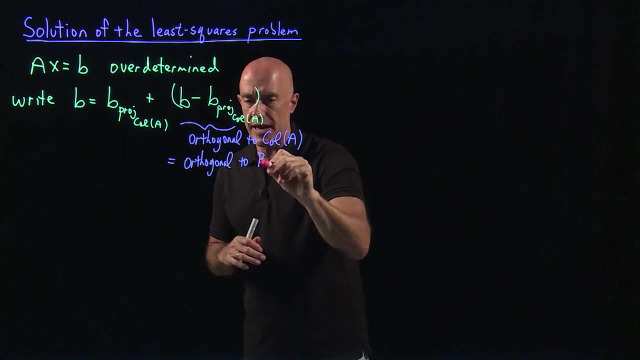 is left over should be orthogonal to the column space of A. So this piece here is orthogonal to the column space of A right. If something is orthogonal to the column space of A, that means It's also orthogonal to the row space of A transpose right, Because the rows of A 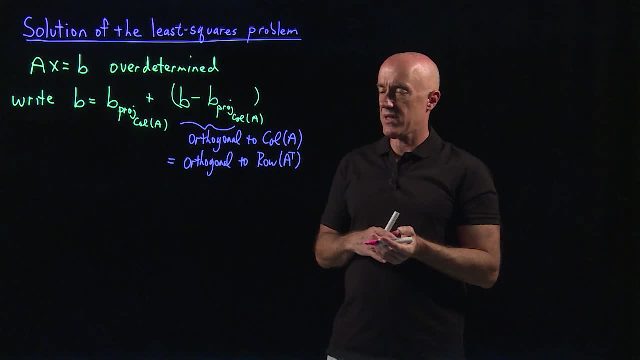 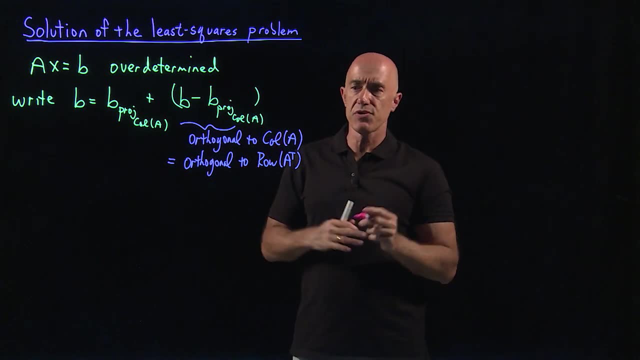 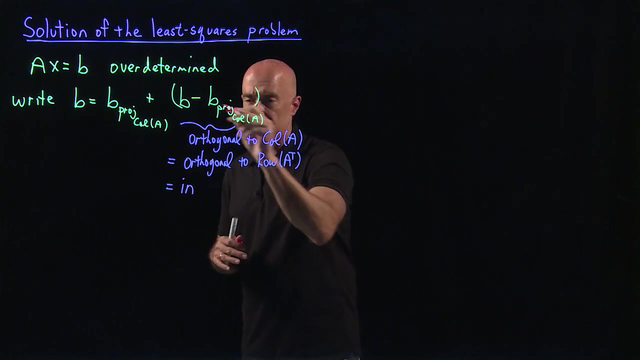 transpose are just the same as the columns of A. Now, a vector that is orthogonal to the rows of a matrix is in the null space of that matrix. So therefore it's in the secant space of that matrix and this vector here is been in the null space of A transpose. 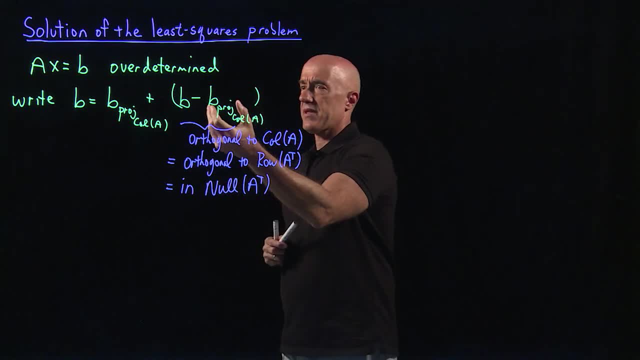 OK, So we write B as a sum of a vector projected onto the B, projected onto the column space of A, plus a vector which is in the null space of A transpose. So to get rid of the vector that's in the null space of A transpose, we just multiply. 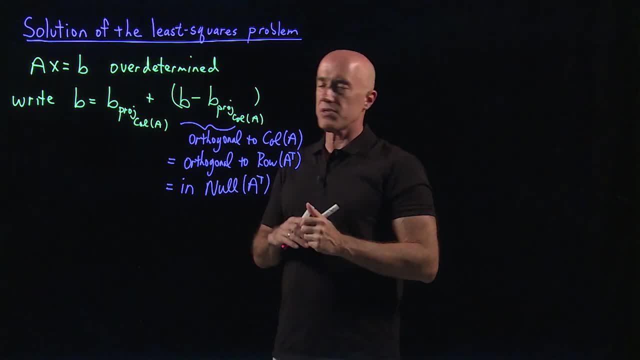 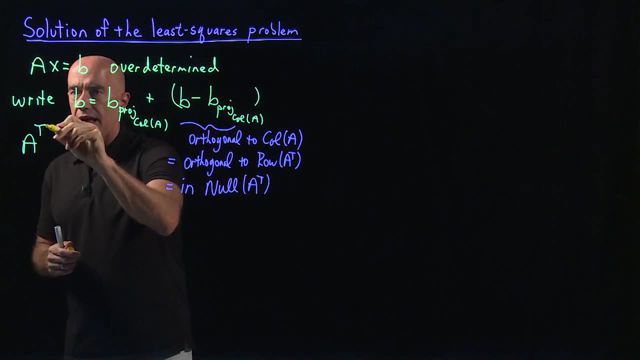 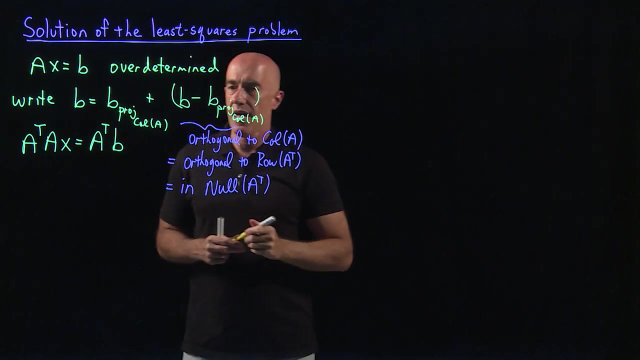 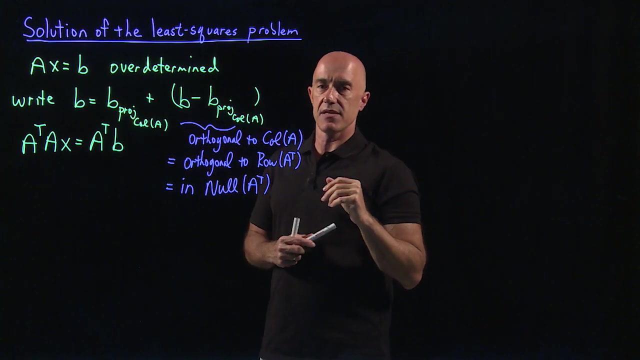 both sides of this equationNetwork- And this is their vectorx- det proposite into constant And those equation by A transpose. So we get A transpose A times X equals A transpose times B. And then when we do that, we multiply by A transpose. then we've gotten rid of the stuff that's. 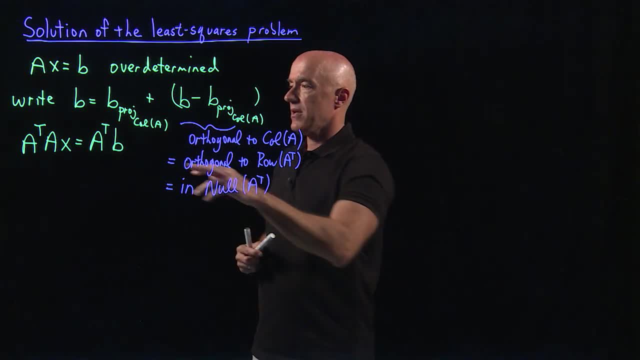 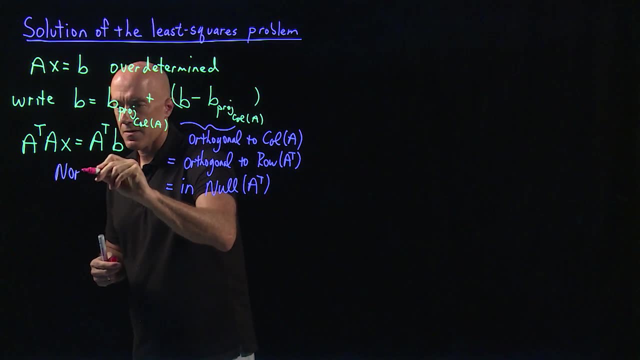 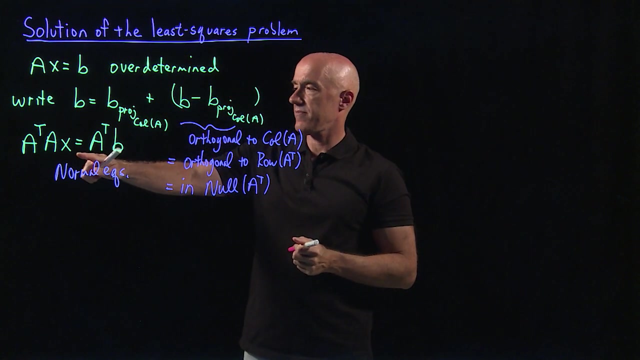 in the null space of A transpose. This system of equations are called the normal equations And in fact these have a solution now for X. And as long as the columns of A are linearly independent, which they are typically in a least squares problem, then you can also show. 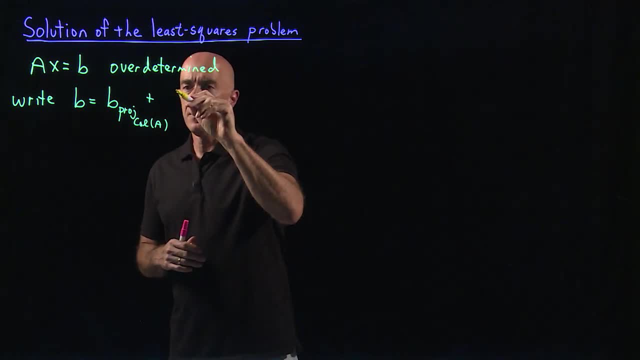 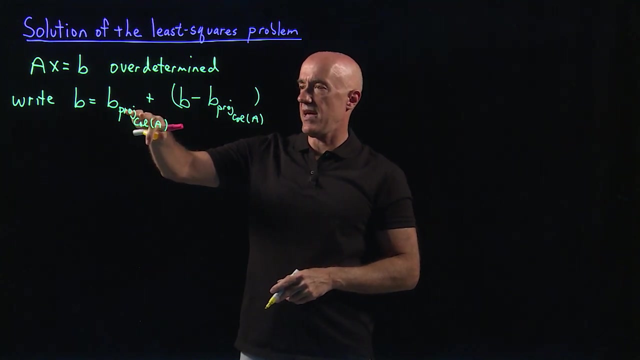 or orthogonal to the column space of A, which we can simply write as: B minus B projected onto the column space of A Right. So B is split into two pieces, One that is projected onto the column space of A plus whatever's left over, So whatever's. 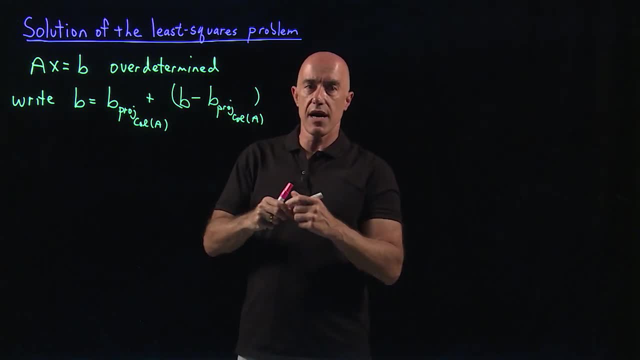 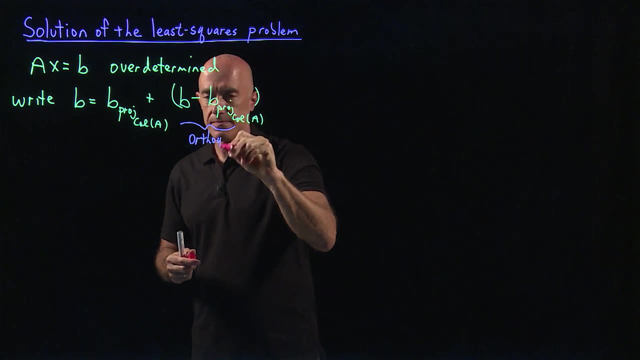 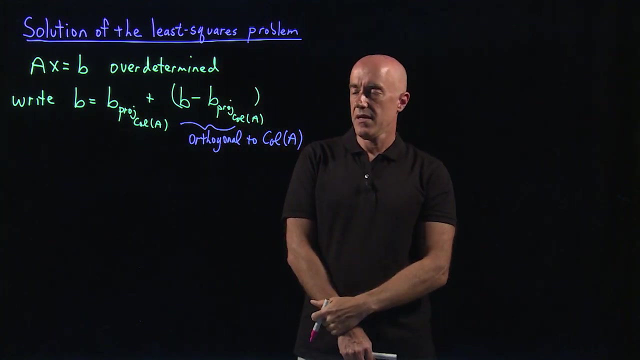 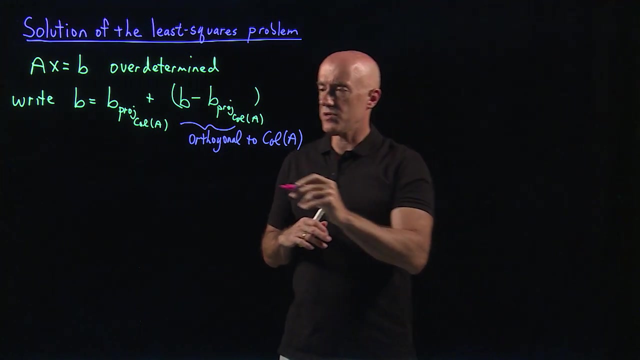 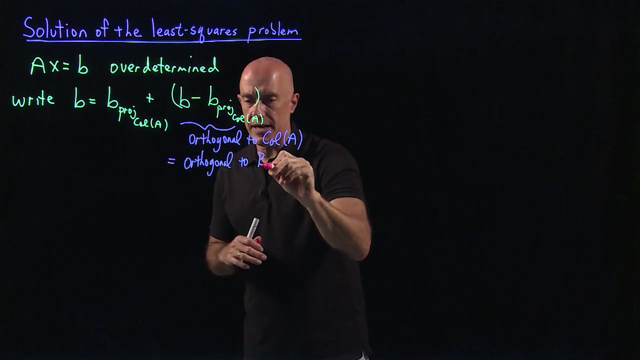 left over should be orthogonal to the column space of A. So this piece here is orthogonal to the column space of A Right. If something is orthogonal to the column space of A, that means It's also orthogonal to the row space of A transpose right. 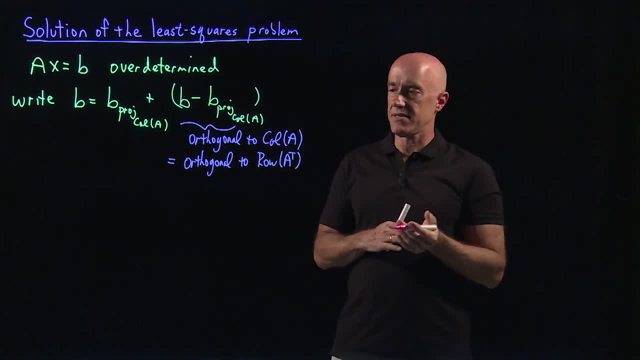 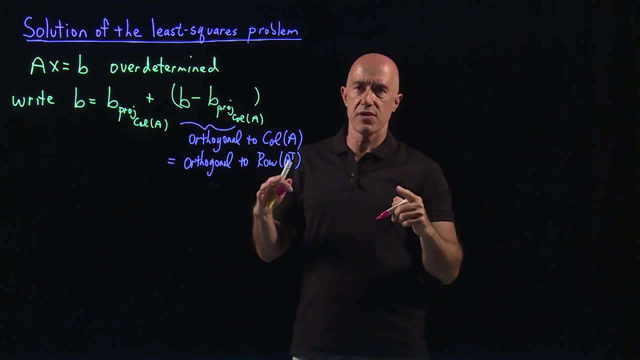 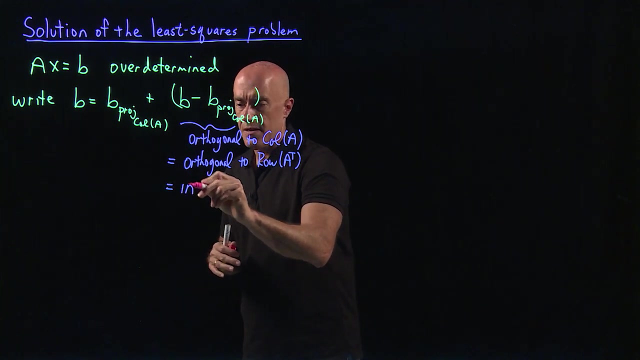 Because the rows of A transpose are just the same as the columns of A. Now a vector that is orthogonal to the rows of a matrix is in the null space of that matrix. So therefore, this vector here is in the null space of A transpose. okay. 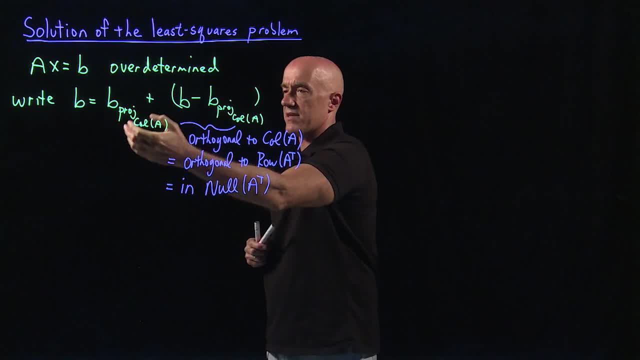 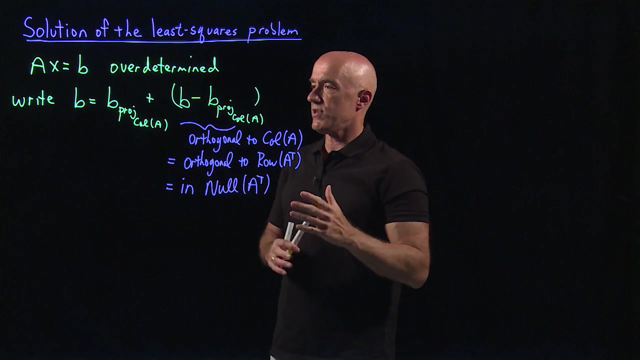 So we write B as a sum of a vector projected onto the column space of A, plus a vector which is in the null space of A transpose, So to get rid of the vector that's in the null space. So to get rid of the vector that's in the null space of A transpose, we just multiply both sides of this equation by A transpose. 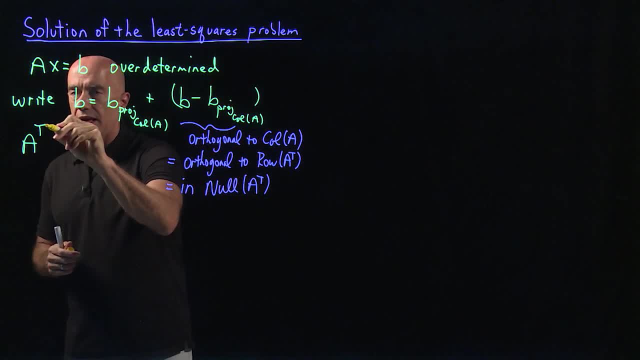 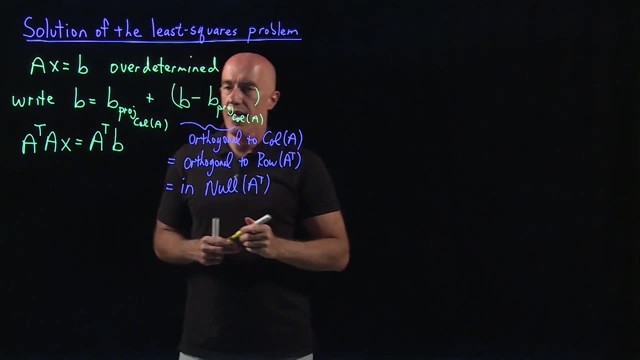 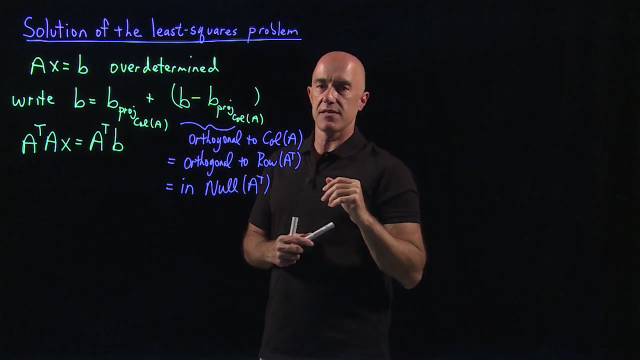 So we get A transpose A times X equals A transpose times B, And then when we do that, we multiply it by A transpose. Then we've gotten rid of the stuff that's in the null space of A transpose. This system of equations. 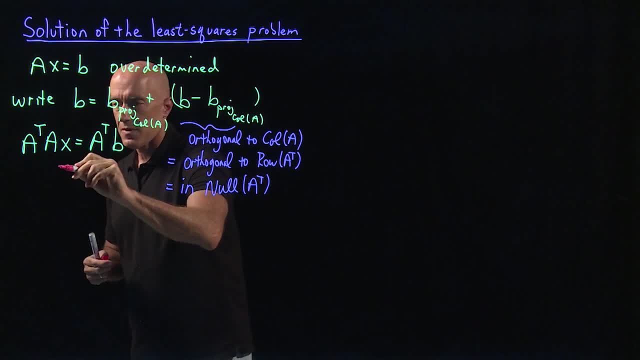 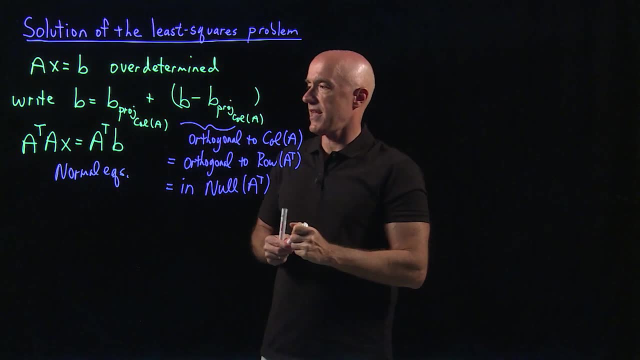 And in fact these have a solution now for X. And as long as the columns of A are linearly independent, which they are typically in a least squares problem, then you can also show that A transpose A is an invertible matrix. So we can. 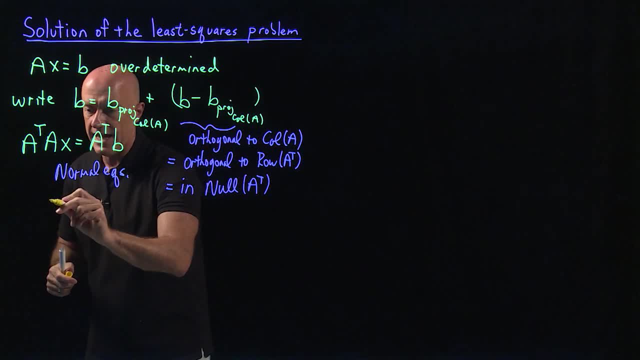 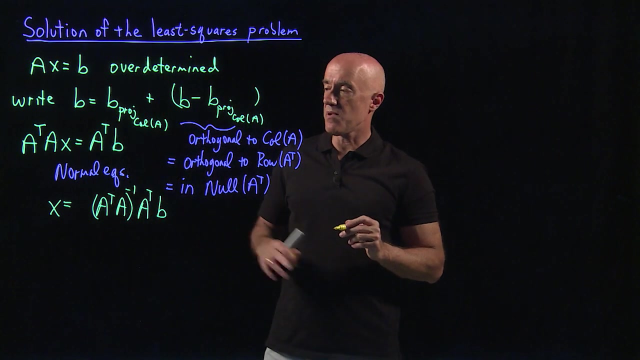 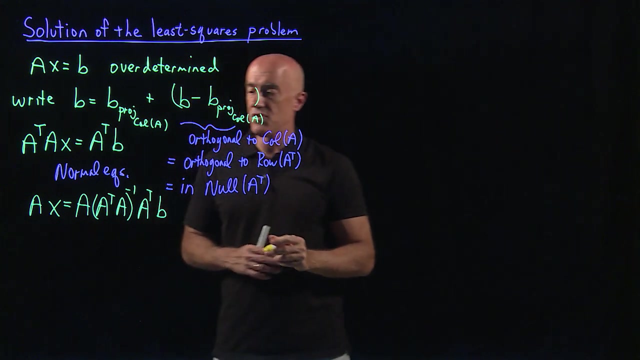 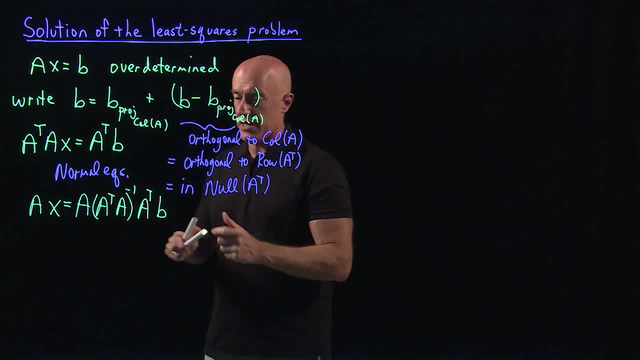 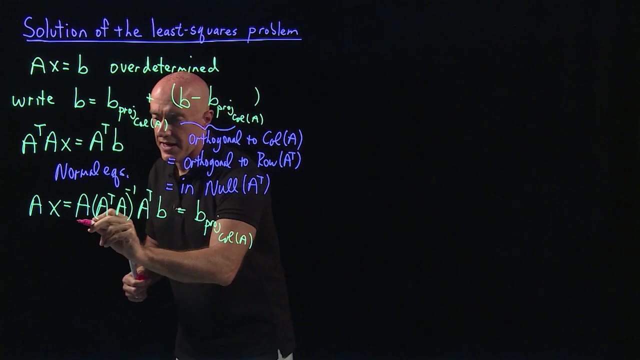 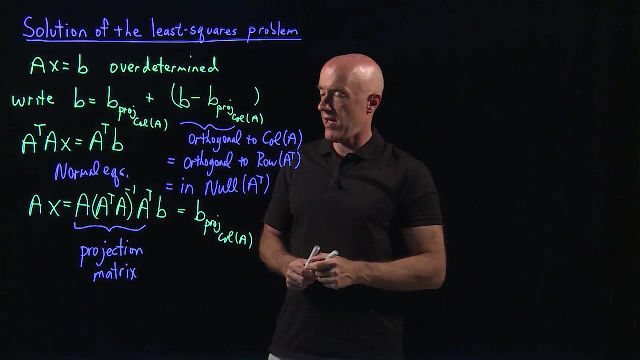 And the right-hand side here is actually equal to the B projected onto the column space of A. So this very fancy-looking matrix here- A times A transpose, A inverse times A transpose- is called a projection matrix. Okay, So that matrix projects B onto the column space of A. 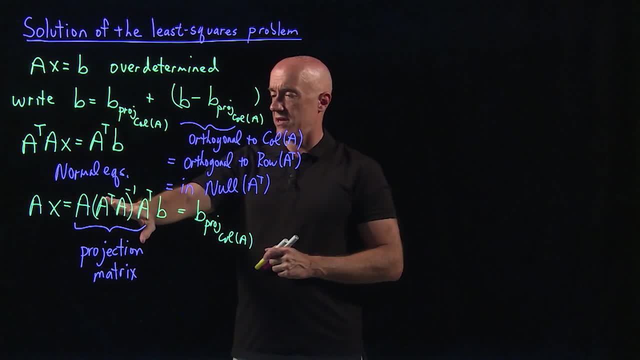 So A is not an invertible matrix, right? If A was an invertible matrix, then you could use the rule of the product of matrices inverse. But A is not even a square matrix, right? A is In the case of the least squares problem. 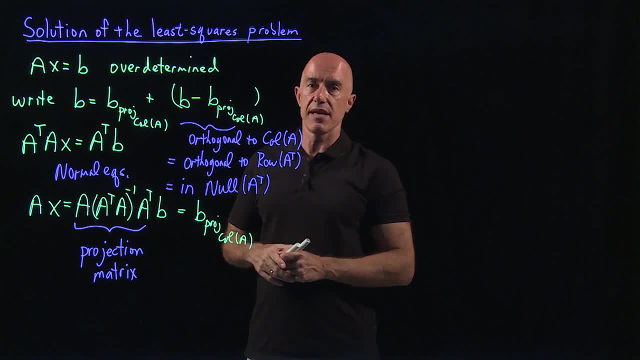 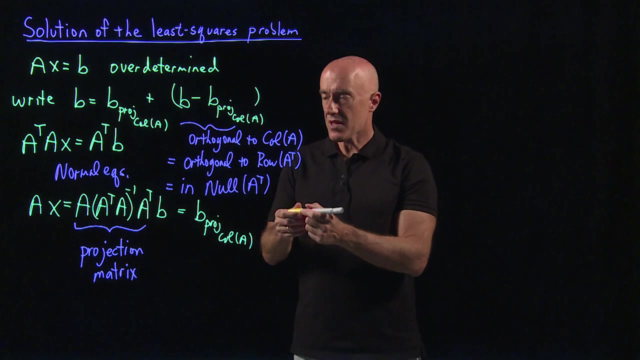 A is a n by 2 matrix, right, But the A transpose A is a square matrix. A transpose A is invertible. And then this quantity, this matrix, here is what's called a projection matrix. Okay, This is just kind of an aside to show you the linear algebra of this problem. 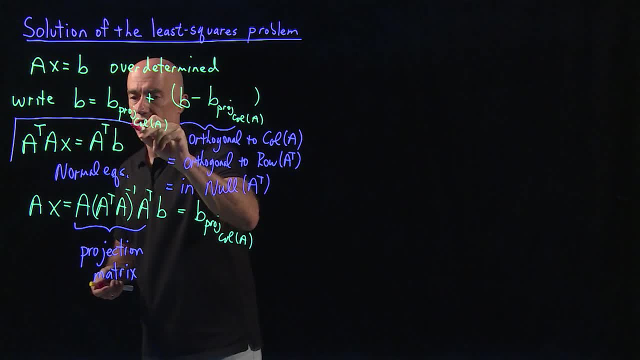 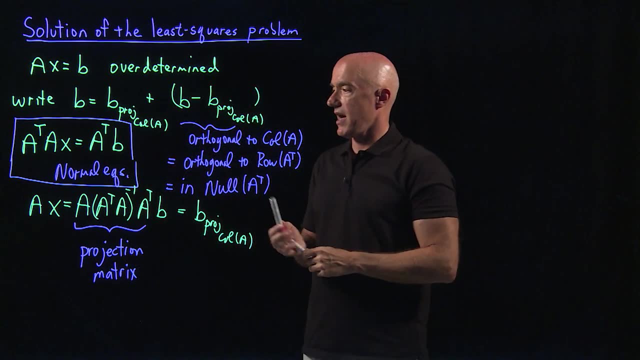 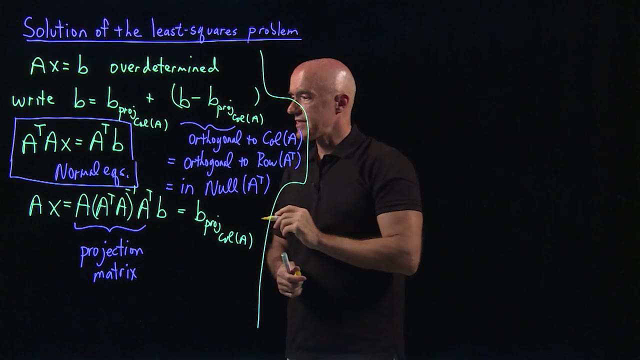 The actual key, though, are these normal equations Right here, And that's what we're going to use to find the least squares line. So let's look at a sample problem, A toy problem. So let's have data. 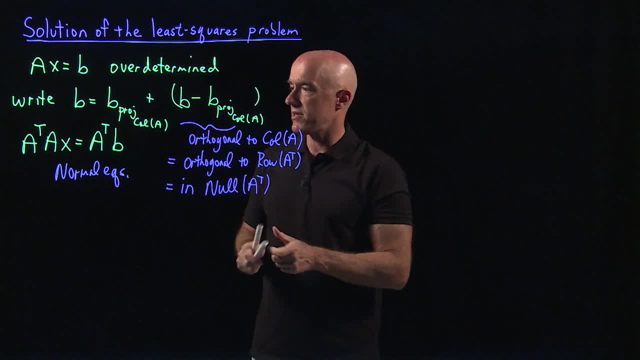 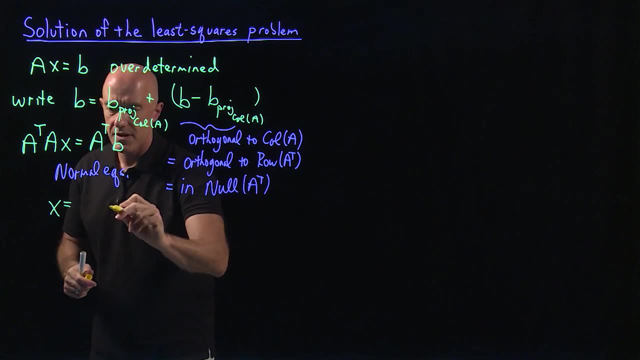 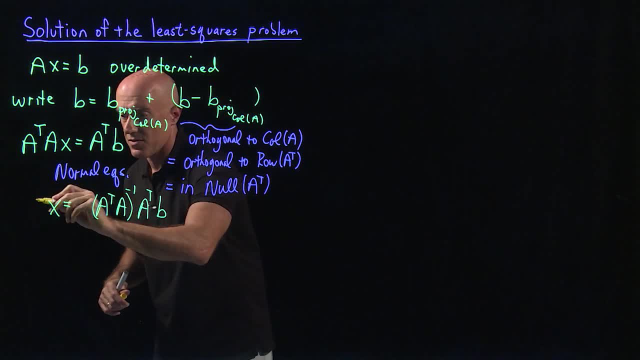 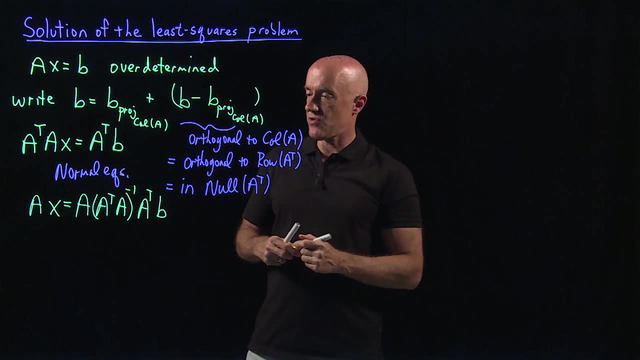 multiply both sides of that equation by A So we could have: AX equals A times A. transpose A inverse times A transpose B, And the right-hand side here is actually equal to X. transpose A, transpose A inverse. when we multiply both sides It's actually a minus. 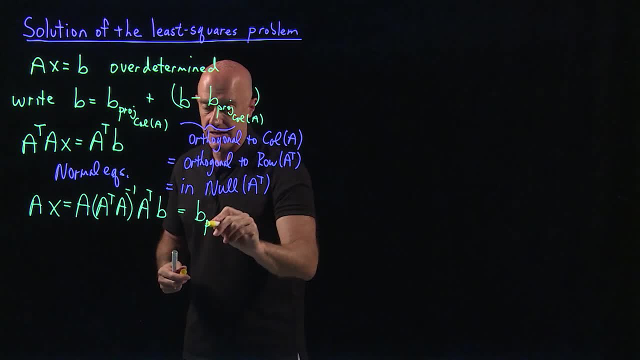 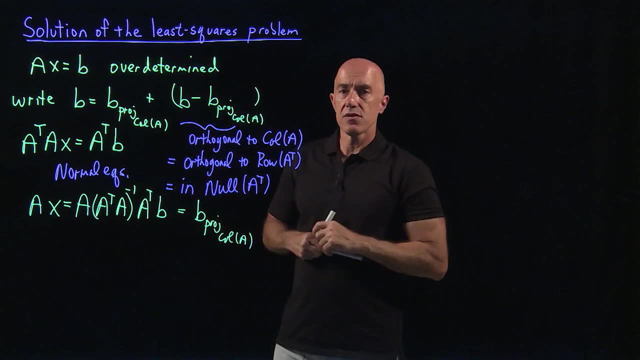 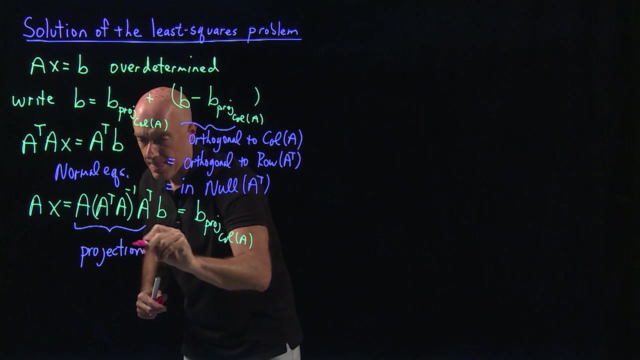 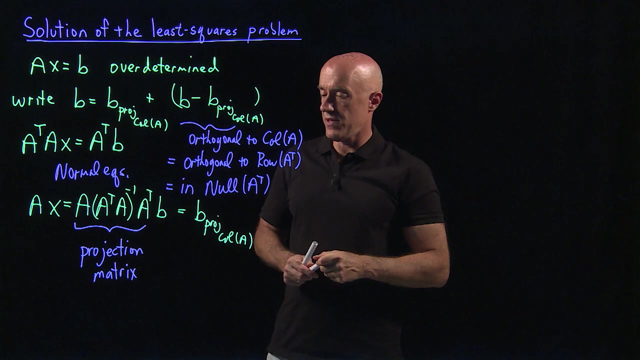 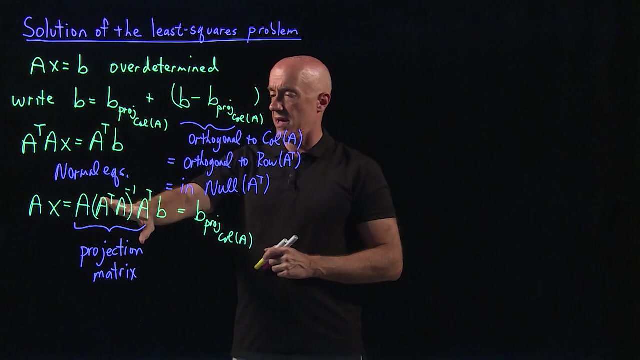 to the B projected onto the column space of A. So this very fancy looking matrix here, A times A transpose, A inverse times A transpose, is called a projection matrix, So that matrix projects B onto the column space of A. So A is not an invertible matrix. If A was an, 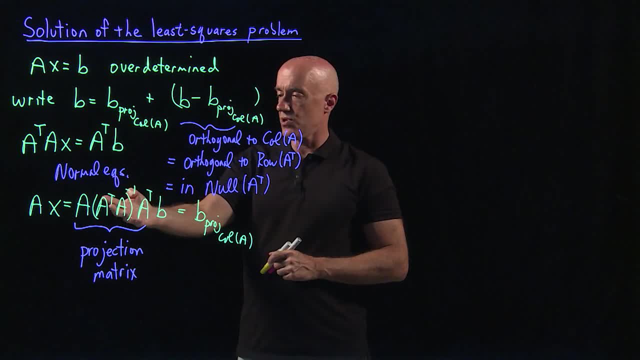 invertible matrix, then you could use the rule of the product of matrices inverse. but A is not even a square matrix. A is, in the case of the least squares problem. A is a n by 2 matrix, But the A transpose A is a square matrix. A transpose A is invertible. And then this: 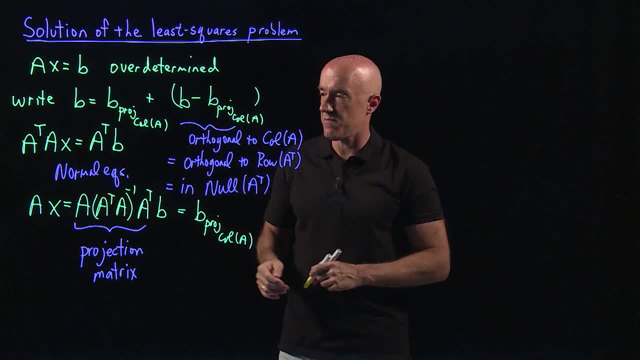 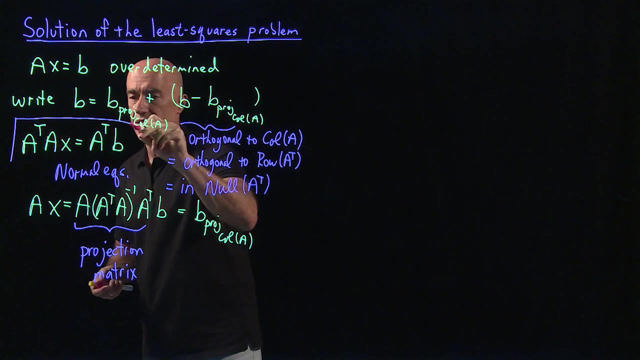 quantity. this matrix here is what's called a projection matrix. This is just kind of an aside to show you the linear algebra of this problem. The actual key, though, are these normal equations right here, And that's what we're going to use to. 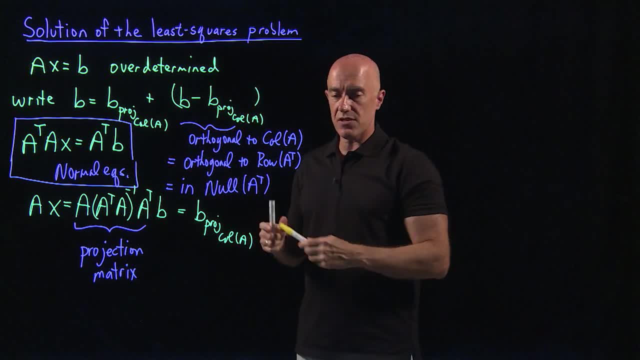 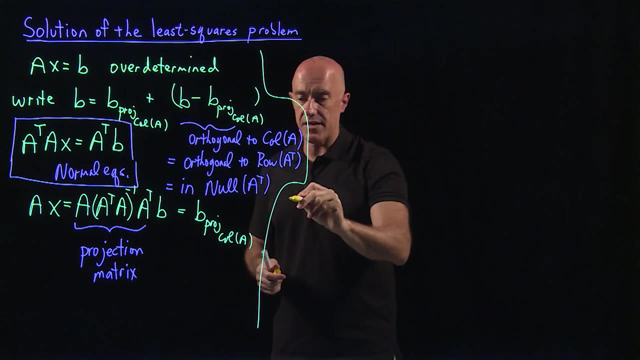 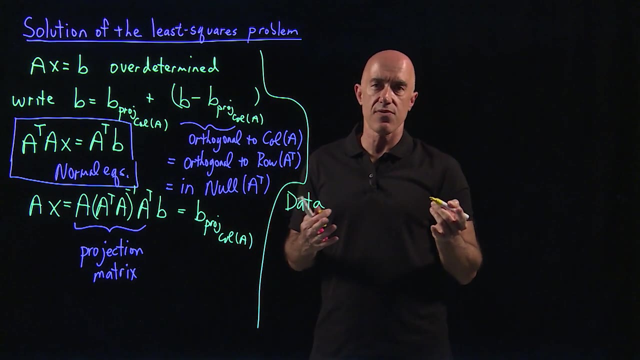 find the least squares line. So let's look at a sample problem, a toy problem. So let's have data. So let's say we have three data points that we want to draw a line through. You know that two points. you can always draw a line through two points. But if you have 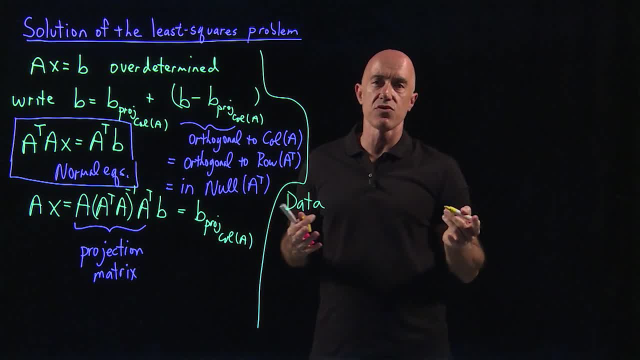 So let's say we have three data points that we want to draw a line through. You know that- two points, You can always draw a line through two points. But if you have three points and they're not collinear, you can always draw a line through two points. 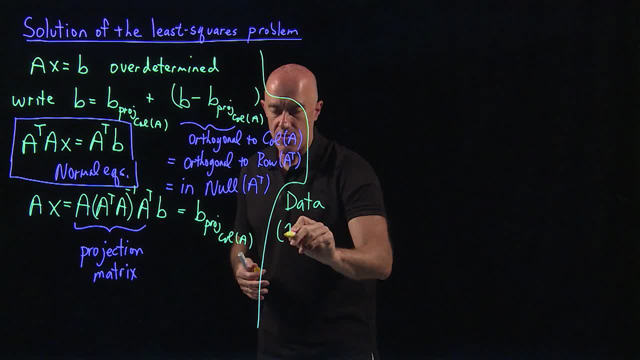 You can't draw a line, So let's have data of three points: 1, 1 will be one of the points, 2, 3 will be the other point, And then the third point will be 3, 2.. 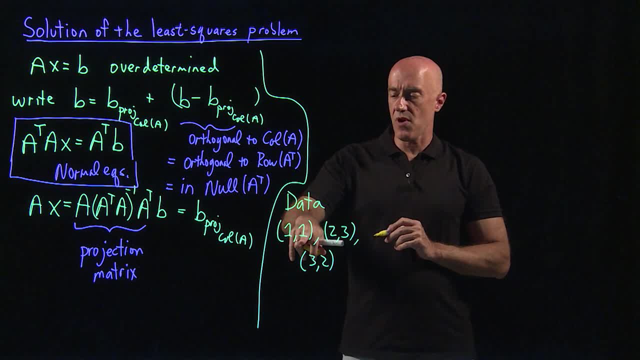 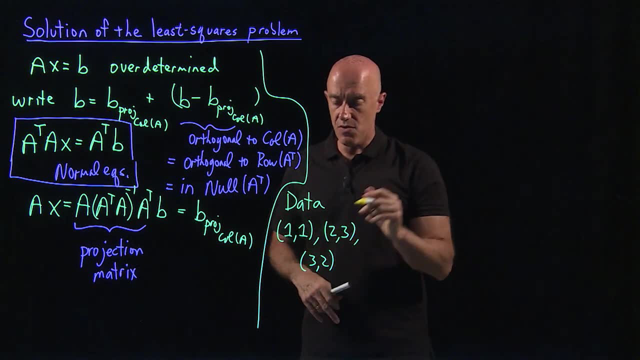 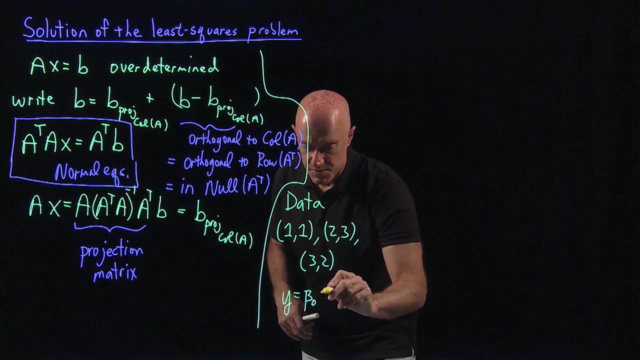 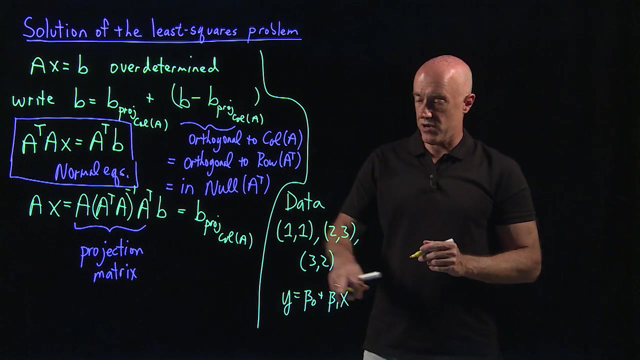 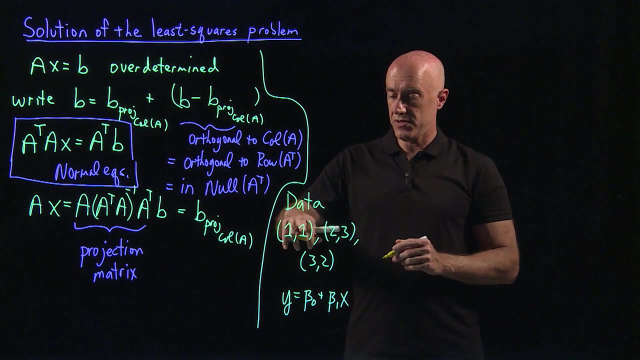 Okay, So let's write down then the equation AX equals B for these points. So we have our line right. We're trying to fit our line: Y equals beta naught plus beta 1X through these three points. So our equation then is the Y, is the Y values. 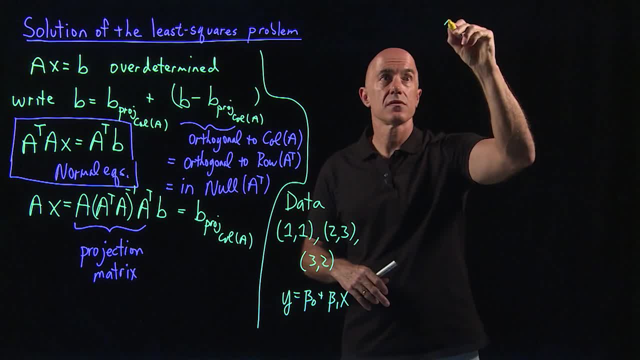 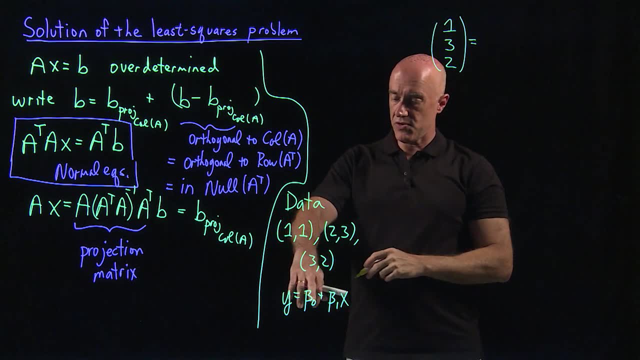 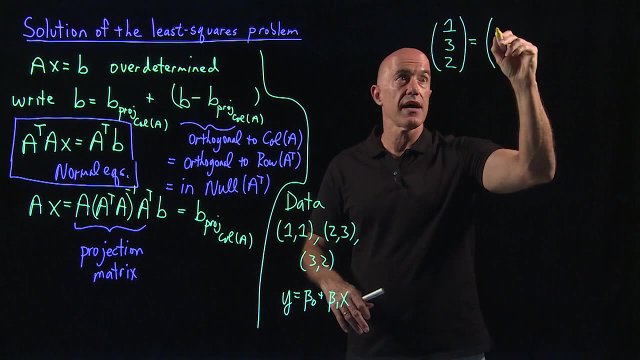 So 1, 3,, 2. Right, And then our matrix. The unknowns are beta naught and beta 1.. And the matrix here is going to be 1 times beta naught plus X1 times beta 1.. 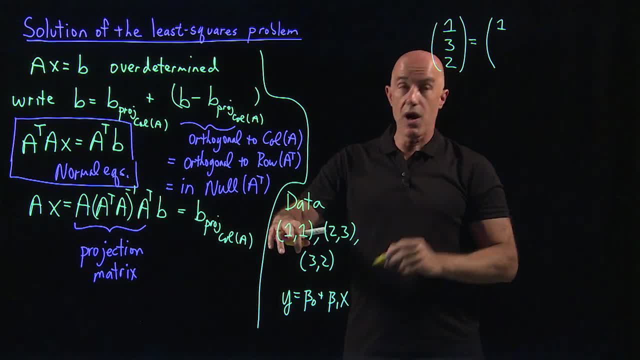 So X1 is going to be 1.. And then 1 times beta naught plus X2 times beta 1. X2 is 2.. And 1 times beta naught times X3 times beta 1. X3 is 3.. 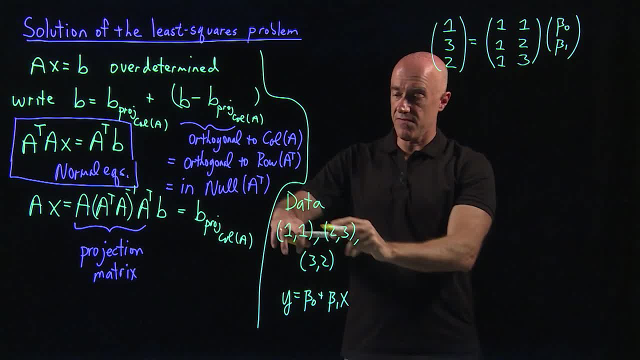 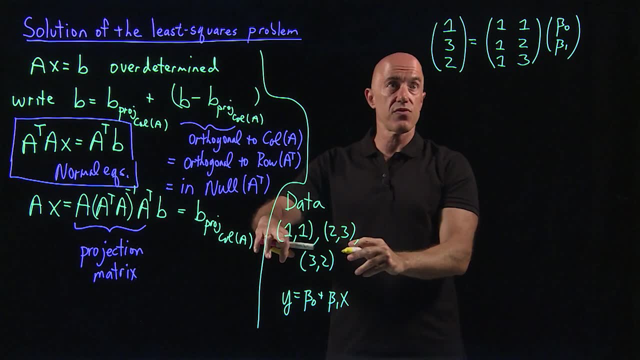 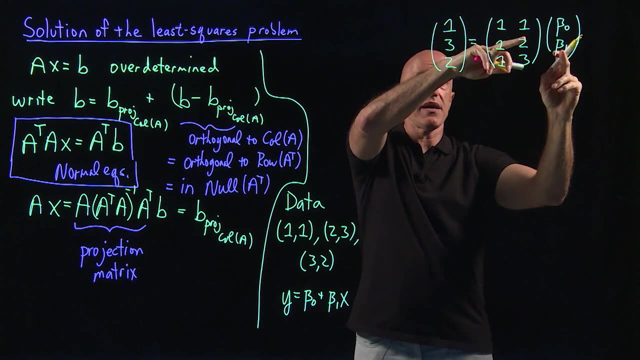 Okay, And that's our system of equations, Trying to fit the line: Y equals beta naught plus beta 1X through these three points. So these are our Y values And then we have beta naught plus 1 times beta 1 equals 1.. 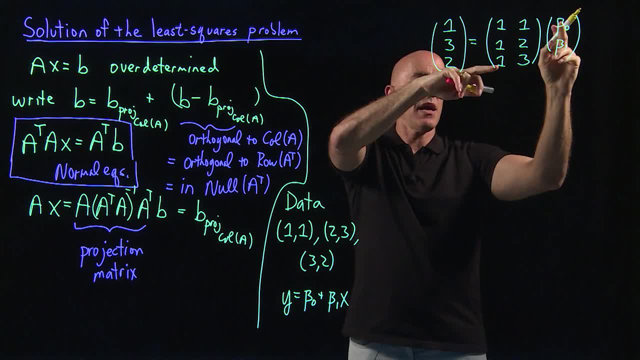 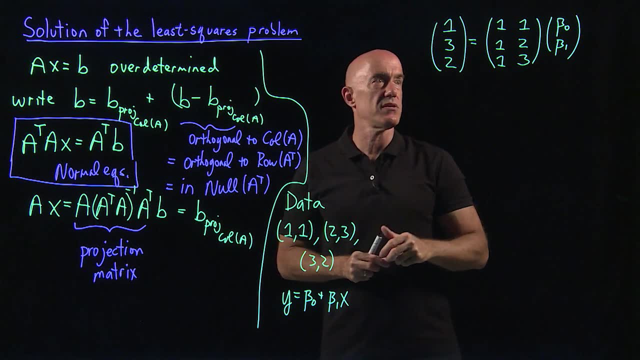 Beta naught plus 2 times beta 1 equals 3.. And beta naught plus 3 times beta 1 equals 2.. So this is an over-determined system of equations. There are three equations and only two unknowns. 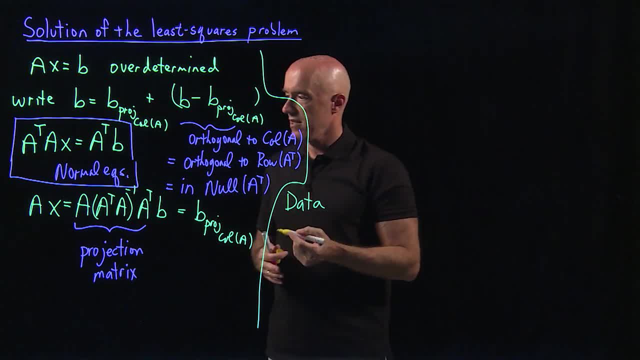 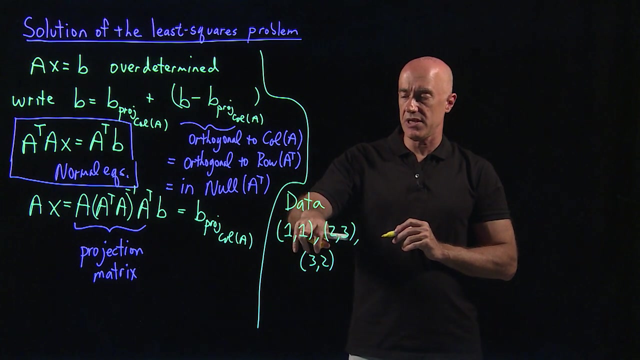 three points and they're not collinear. you can't draw a line. So let's have data of three points: One, one will be one of the points, Two, three will be the other point, And then the third point will be three, two, OK, So let's write down then the equation: Ax equals. 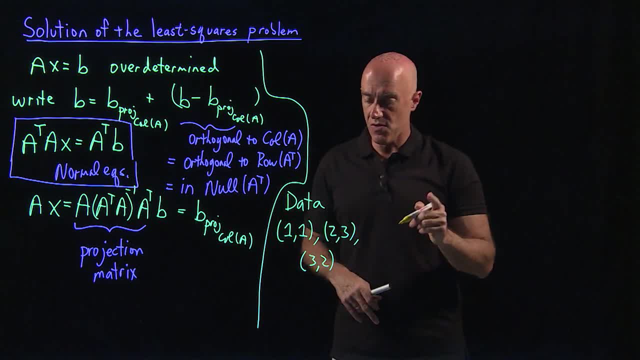 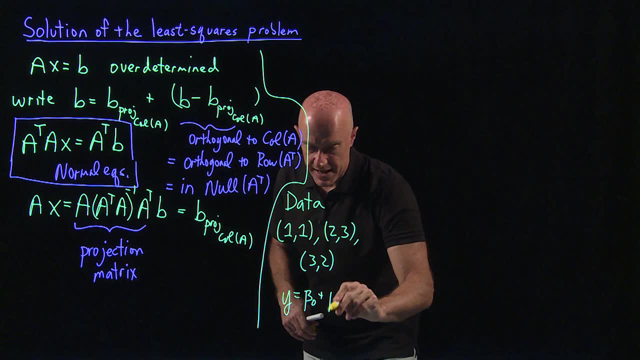 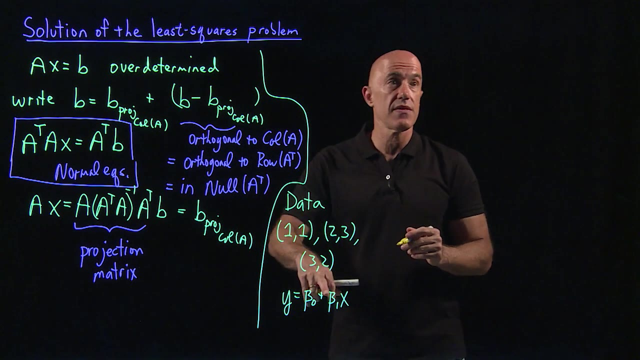 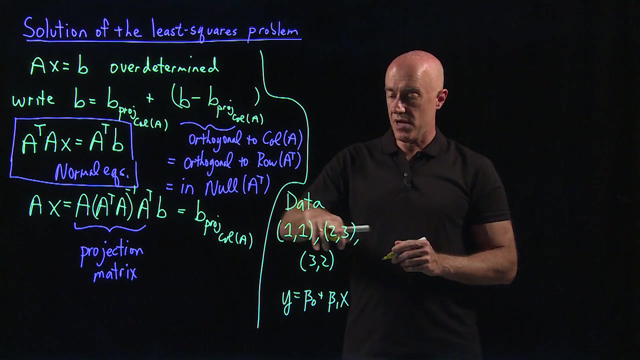 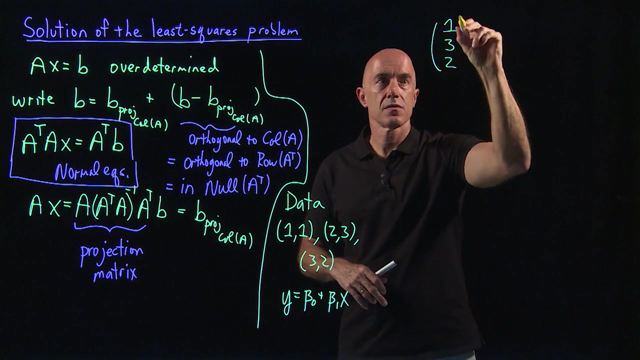 B for these points. So we have our line right. We're trying to fit our line. y equals beta naught plus beta 1x through these three points. So our equation then is the y is the y values. so 1,, 3, 2, right. 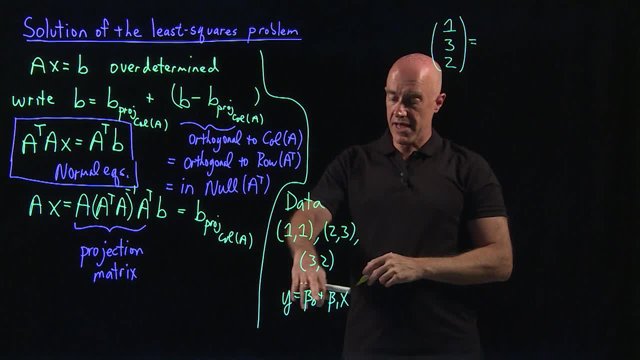 And then our matrix. the unknowns are beta naught and beta 1.. And the matrix here is going to be 1 times beta naught plus x1 times beta 1.. So x1 is going to be 1.. And then 1 times beta naught plus x2 times beta 1, x2 is 2.. 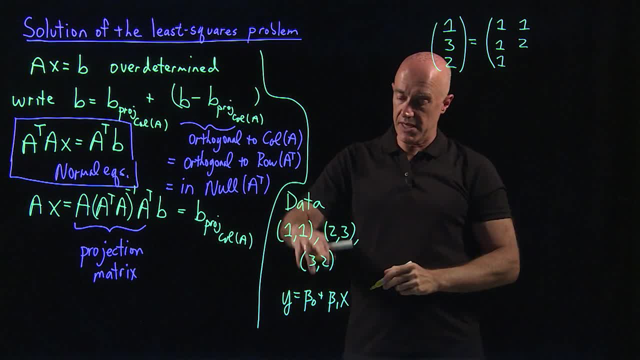 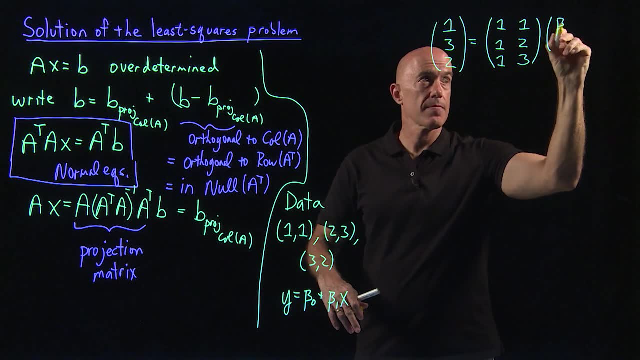 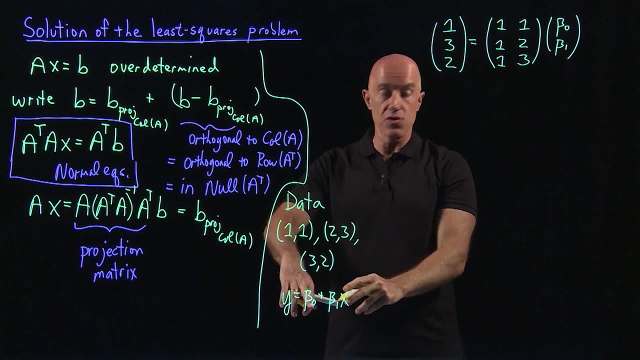 And 1 times beta naught times x3 times beta 1.. X3 is 2.. And 1 times beta naught plus x2 times beta, 1 is 3.. And that's our system of equations. trying to fit the line y equals beta naught plus. 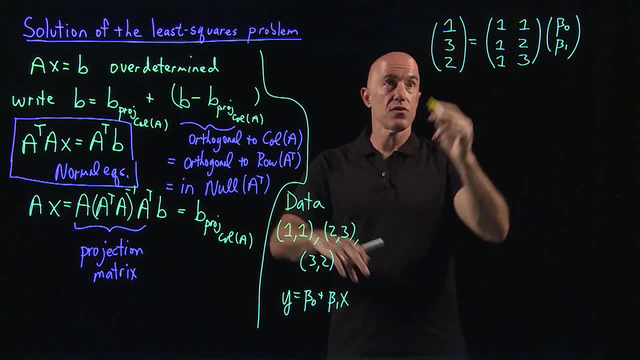 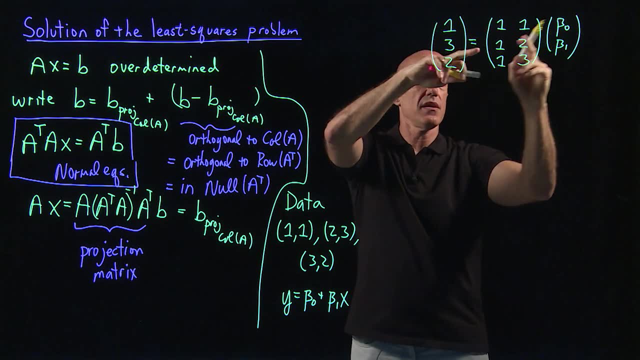 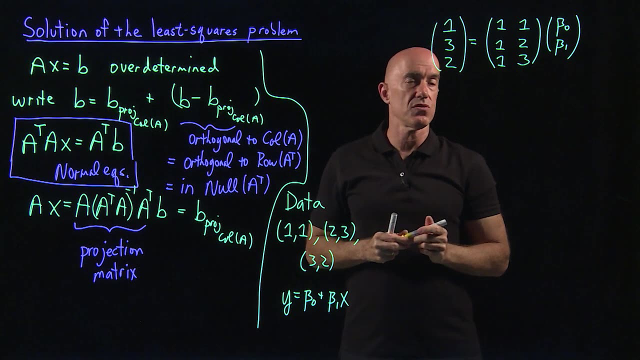 beta 1x through these three points. So these are our y values. And then we have beta naught plus 1 times beta 1 equals 1, beta naught plus 2 times beta 1 equals 3, and beta naught plus 3 times beta 1 equals 2.. 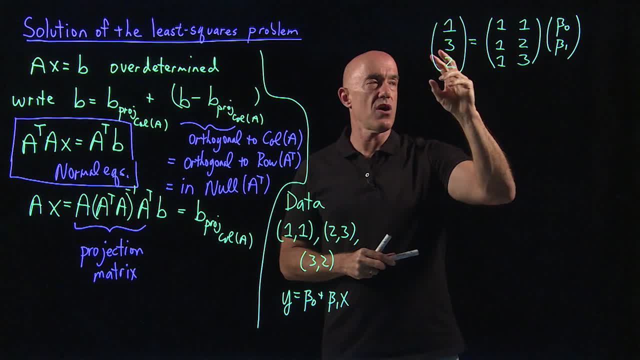 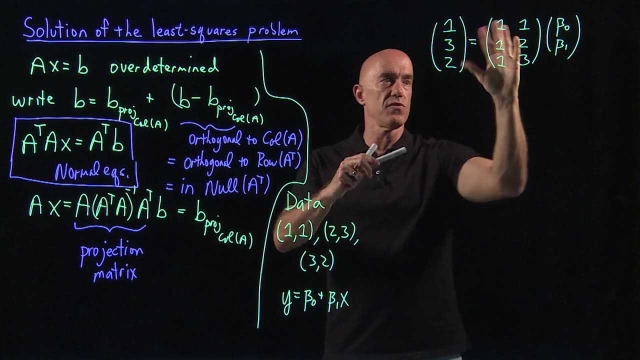 This is an overdetermined system of equations. There are three equations and only two unknowns. The points are not collinear, so there's no solution. So to solve this, then we form the normal equations. So the normal equations. if you allow me to flip the order, because I'm so used to writing. 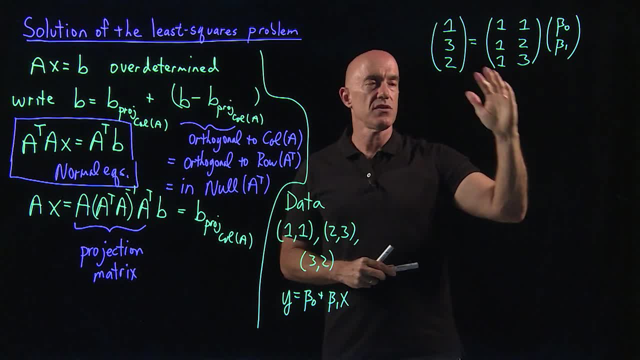 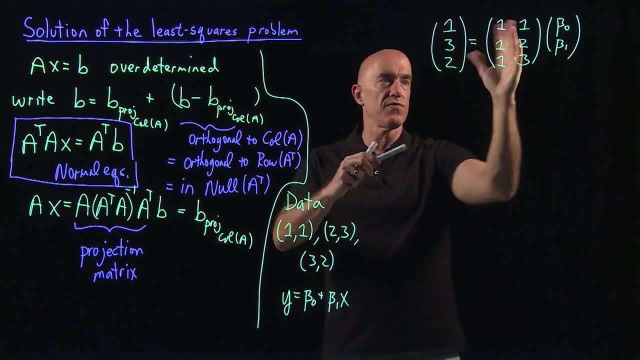 The points are not collinear, So there's no solution. So to solve this, then we form the normal equations. So the normal equations, if you allow me to flip the order, because I'm so used to writing: AX equals B. 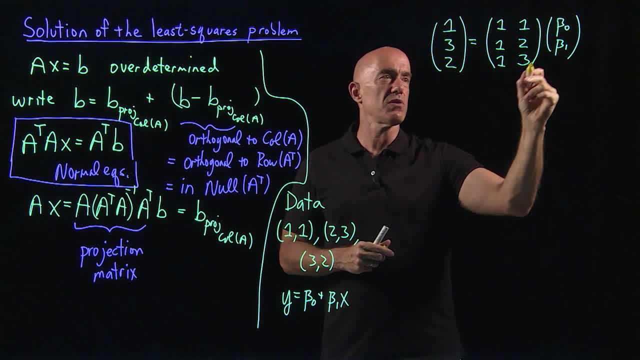 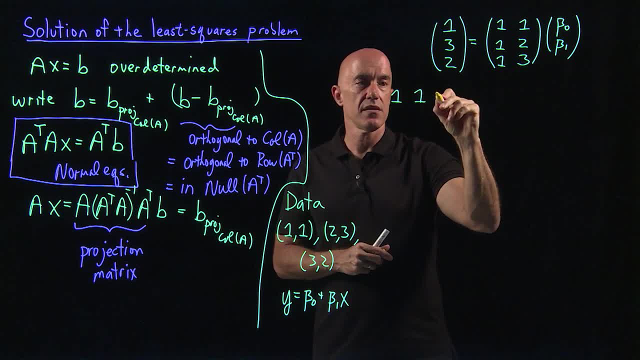 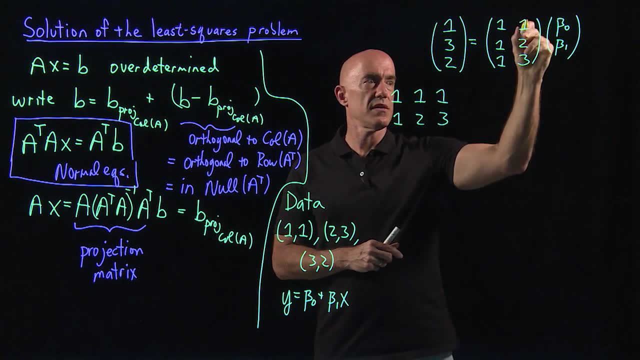 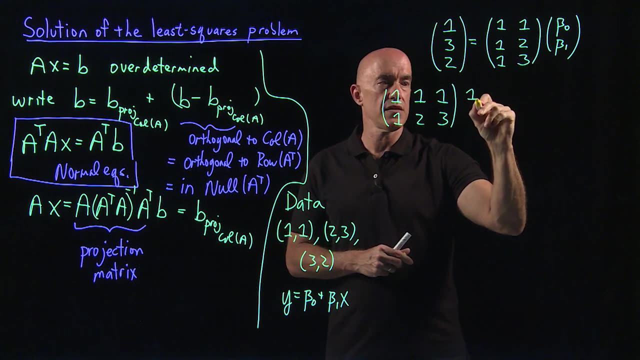 Okay, So we have A transpose is 1, 1, 1,, 1,, 2, 3.. The first column becomes the first row, The second column becomes the second row. So A transpose times A, which is 1, 1,, 1,, 2,, 1, 3.. 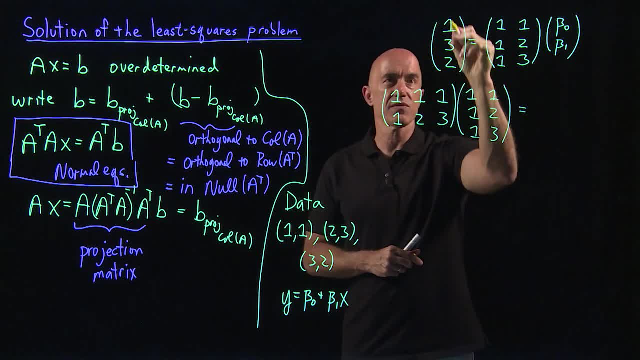 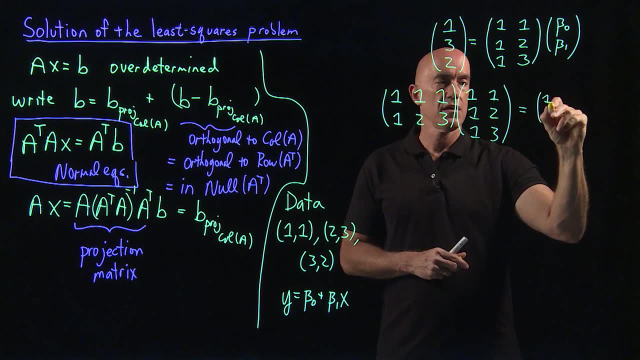 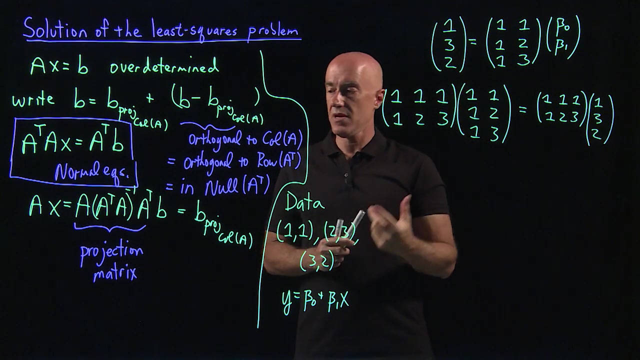 A transpose times A equals A transpose times Y, so that will be A transpose times Y. so we have 1, 1, 1, 1, 2, 3 times Y, which is 1, 3, 2.. So this is the normal equations. A transpose times A equals A transpose. 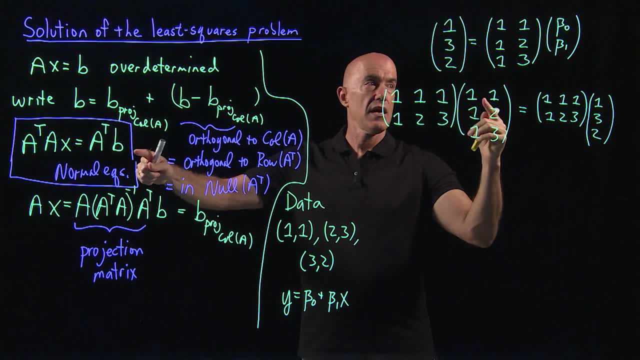 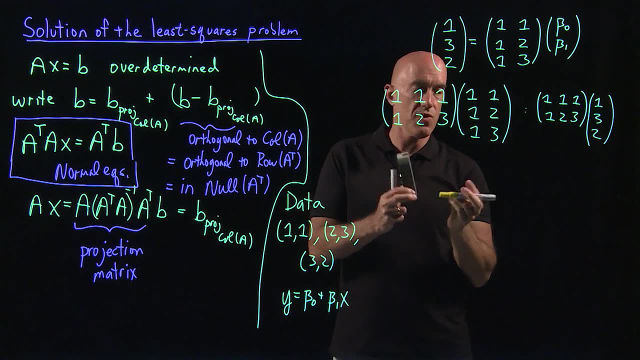 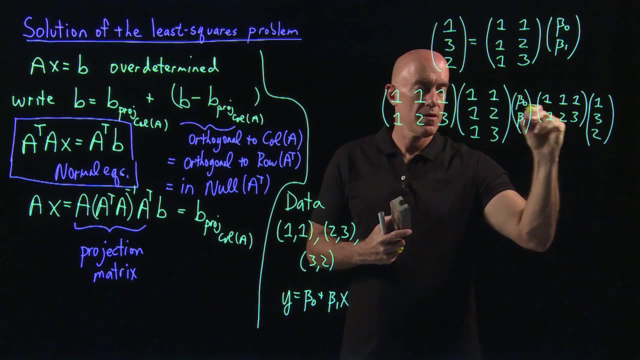 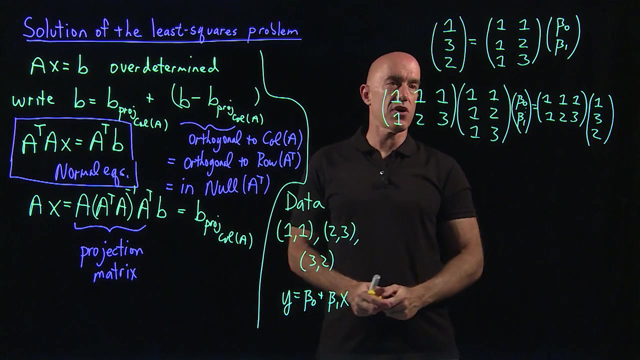 times A transpose A times X. sorry, A transpose A times X, which is our beta 0, beta 1, equals A transpose times B. Okay, Those are our normal equations, So we can do a little bit of arithmetic here. 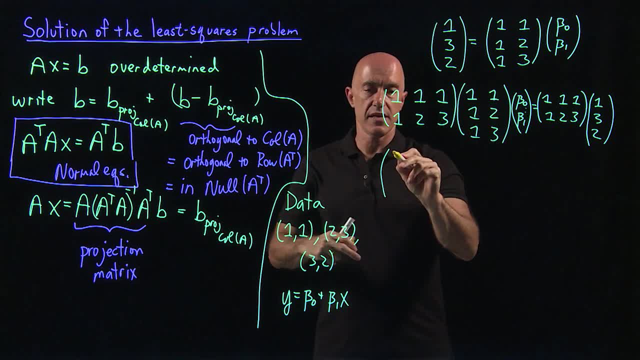 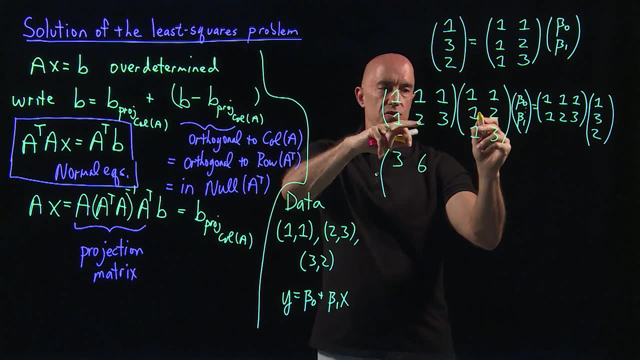 So we have: 1 plus 1 plus 1 is 3,, 1 plus 2 is 3 plus 3 is 6,. 1 plus 2 plus 3 is 5, 6, and 1 plus 4 is 5 plus 9 is 14.. 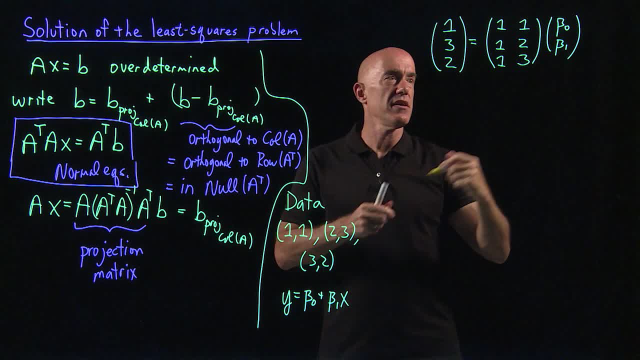 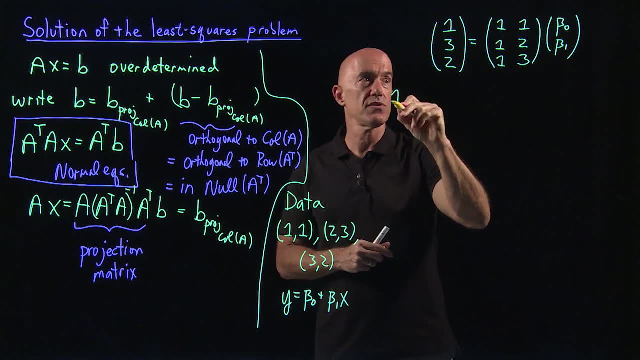 ax equals b. let me change the order here. The normal equations multiplies both sides by a transpose. So we have a transpose is 1, 1, 1, 1, 2, 3.. The first column becomes the first row. 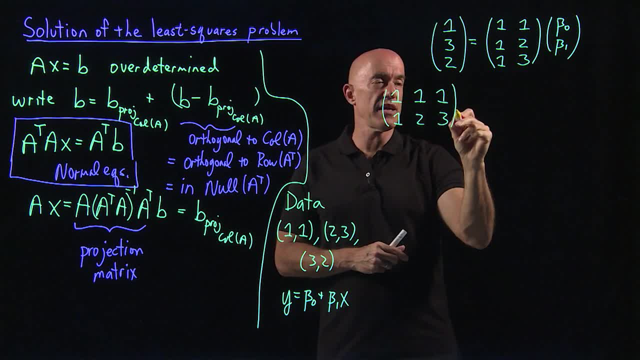 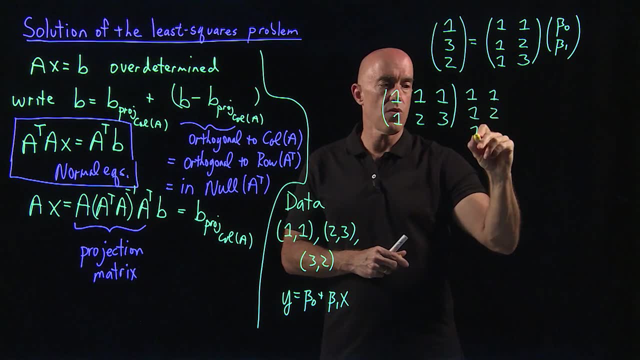 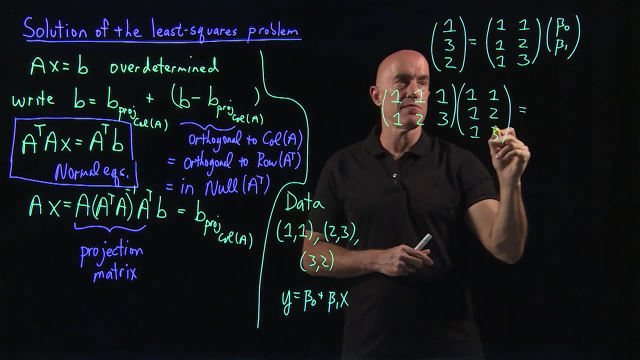 The second column becomes the second row, So a transpose times a, which is 1, 1, 1, 2, 1, 3.. A transpose times a equals a transpose times y, So that will be A transpose times y. 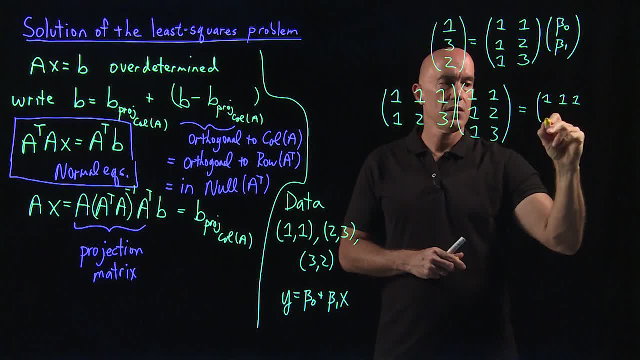 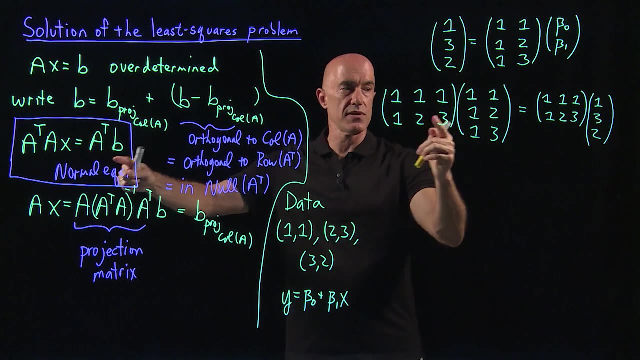 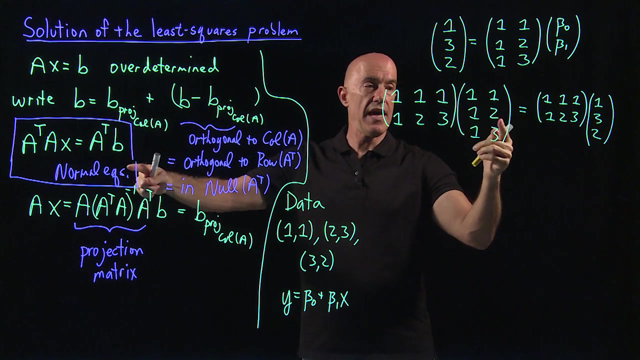 So we have 1, 1, 1, 1, 2, 3 times y, which is 1, 3, 2.. So this is the normal equations. A transpose times A equals A transpose times A transpose A times x. sorry, 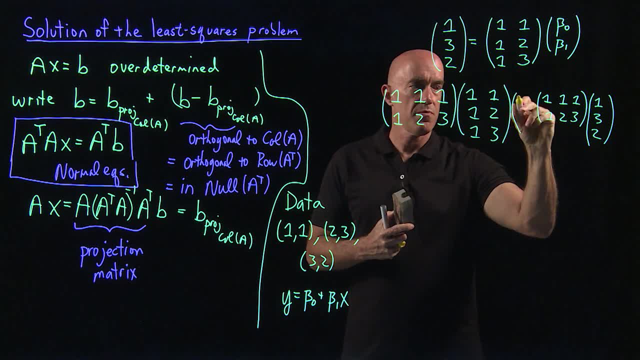 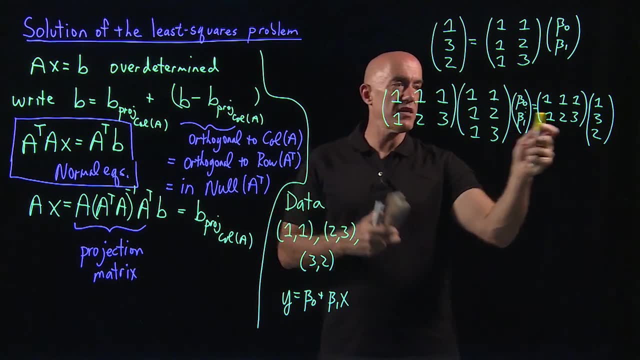 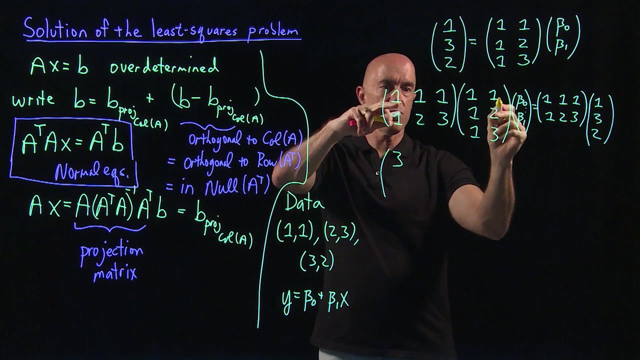 A transpose A times x, which is our beta 0, beta 1, equals A transpose times B. Those are our normal equations. Okay, So we can do a little bit of arithmetic here. So we have: 1 plus 1 plus 1 is 3,. 1 plus 2 is 3 plus 3 is 6,. 1 plus 2 plus 3 is 5, 6.. 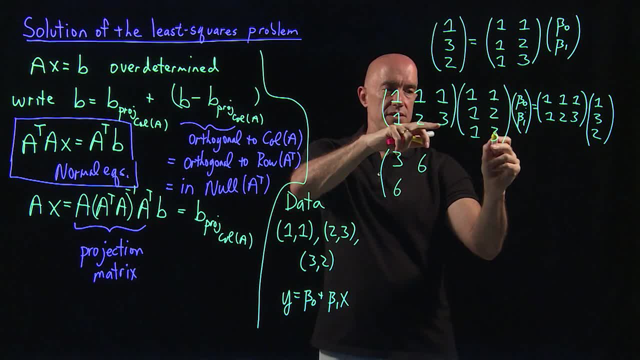 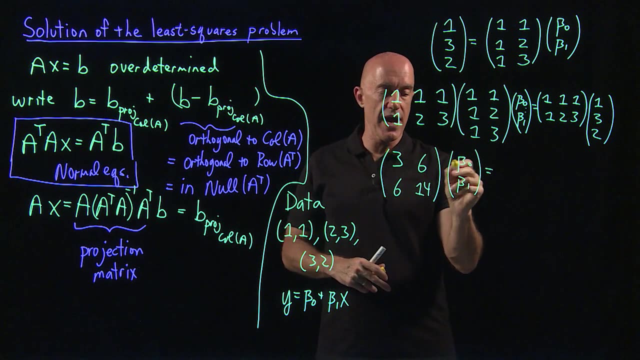 And 1 plus 4 is 5 plus 9 is 14.. So this becomes a 2 by 2 matrix. This becomes beta 0, beta 1, our unknown vectors, the y-intercept and the slope of the line. 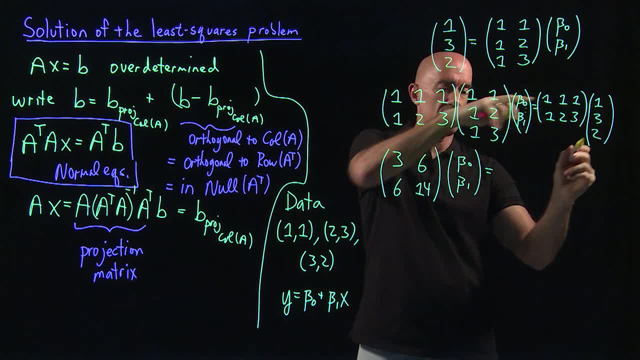 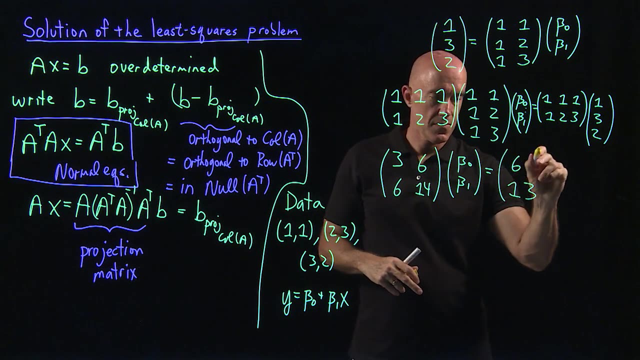 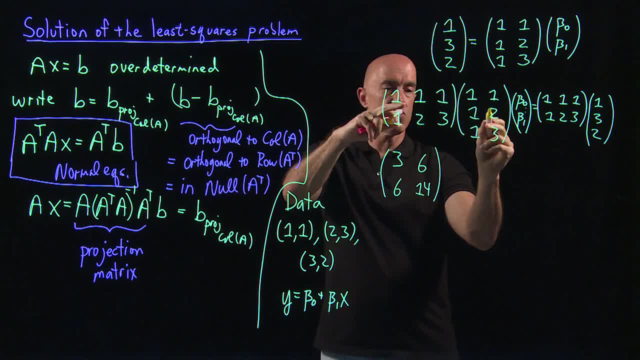 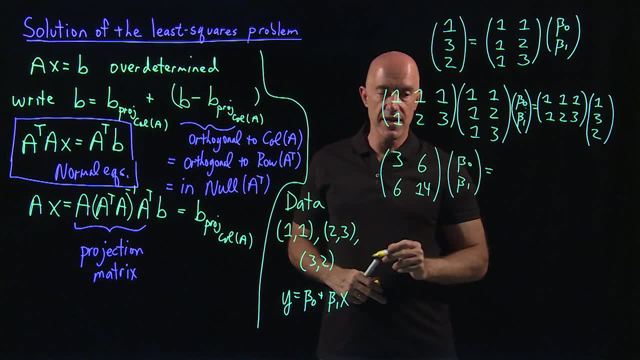 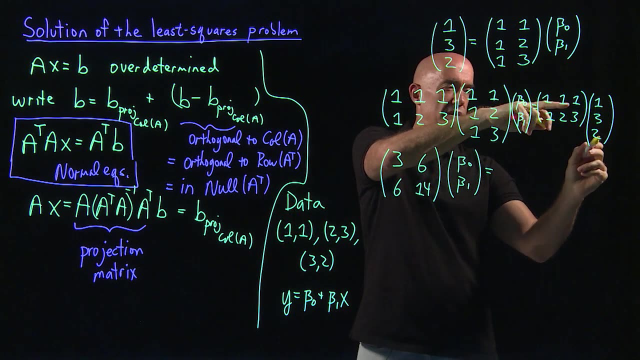 So this becomes a 2 by 2 matrix times beta naught beta 1, our unknown vectors, the y-intercept and the slope of the line, And the right-hand side then is 1 plus 3 plus 2 is 6, and 1 plus 6 is 7 plus 6 is 13.. 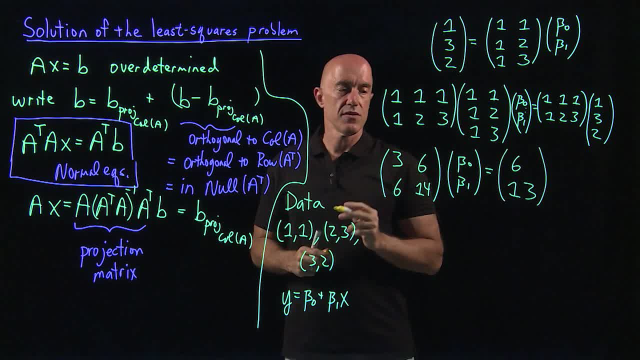 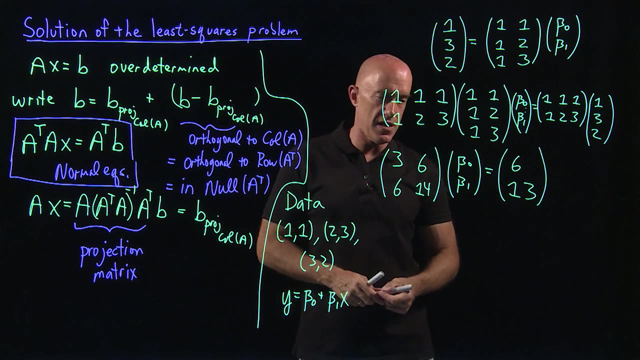 Okay, So these are the normal equations: the A transpose A, X equals A transpose B, So this is solvable, right? This is a system of two equations and two unknowns. We can use any method to solve this, including Gaussian elimination, but it's only a 2 by 2 system. 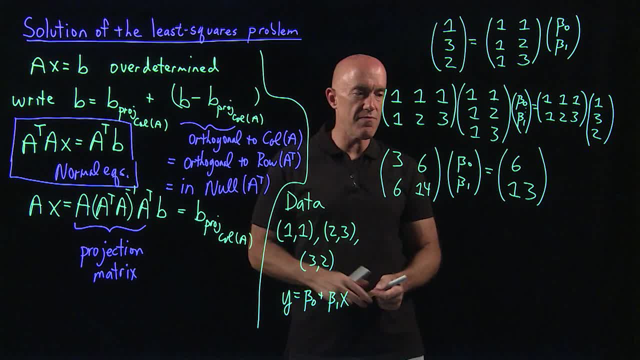 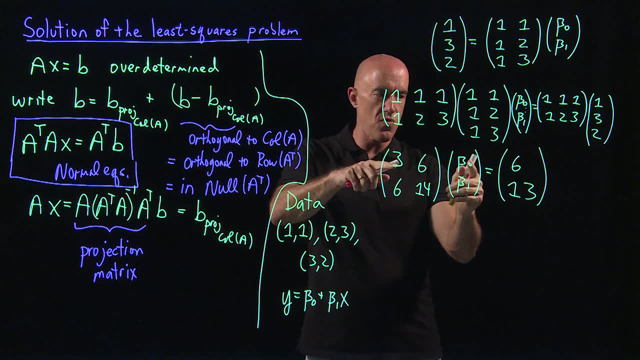 Or you can see what the solutions are. I have my solutions written down, I have my solution over there, but let me kind of guess it here. I think beta naught is 1 and beta 1 is a half. So 3 plus 3 is 6, and 6 plus 7 is 13.. 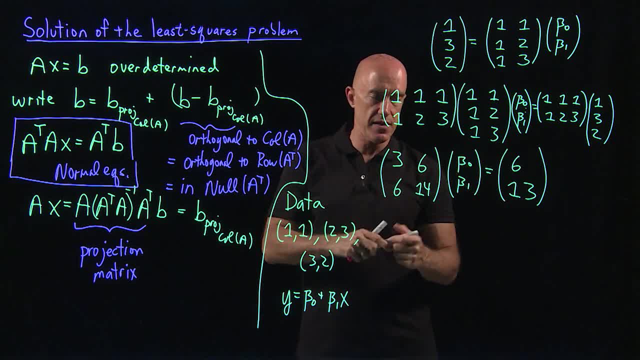 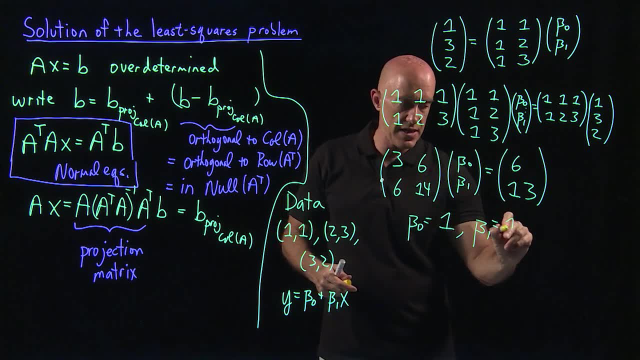 So beta naught 1, 1 half will solve this right. So this solution is: beta naught equals 1 and beta 1 equals 1 half. Very nice numbers, because I set up the problem So that the numbers are nice. 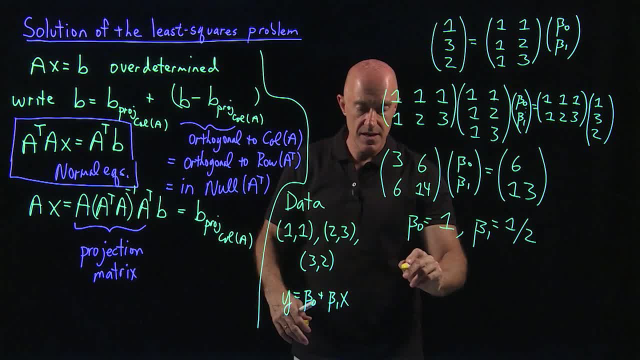 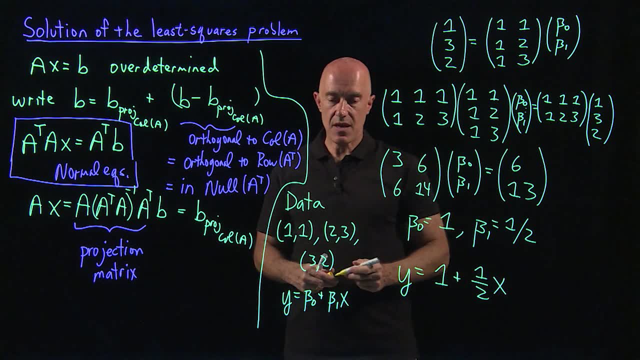 So the best fit line then here is our: Y equals 1 plus 1 half X, And that's the best fit line for these data points. Okay, If you look at the notes, you'll see the graph and get an idea of how good this is. 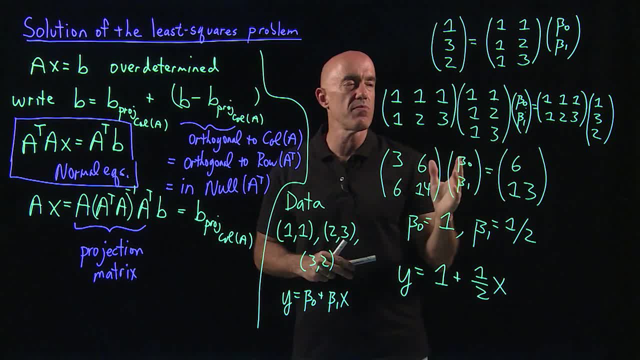 So this is just a toy problem, one I can work on the board. So we only have three data, Okay, But typically in a least squares fit. you have a large number of data that you're trying to fit a line through, So let me review. 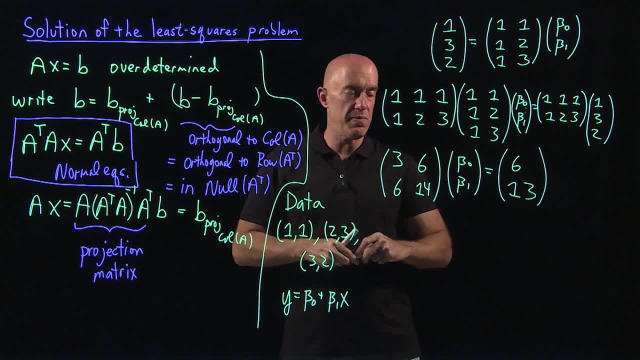 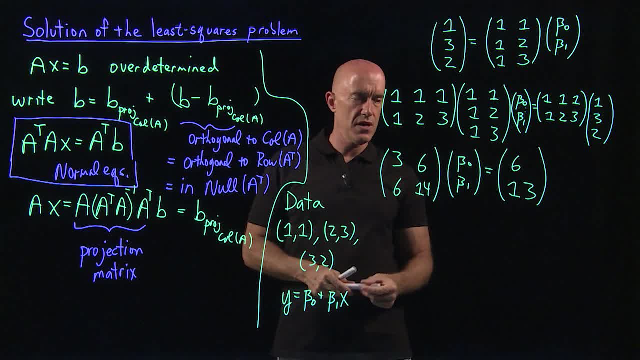 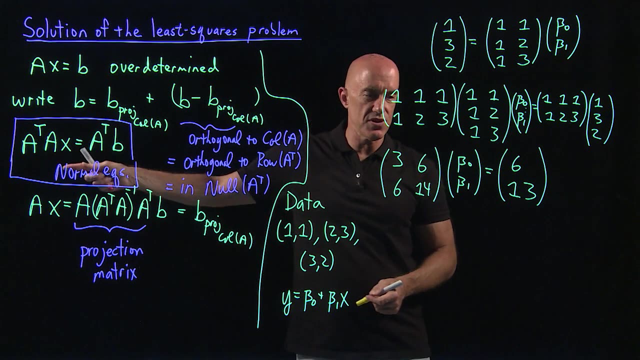 This is a system of two equations and two unknowns. We can use any method to solve this, including Gaussian elimination, but it's only a 2 by 2 system. Or you can see what the solutions are. I have my solutions written over there, but let me kind of guess it here. 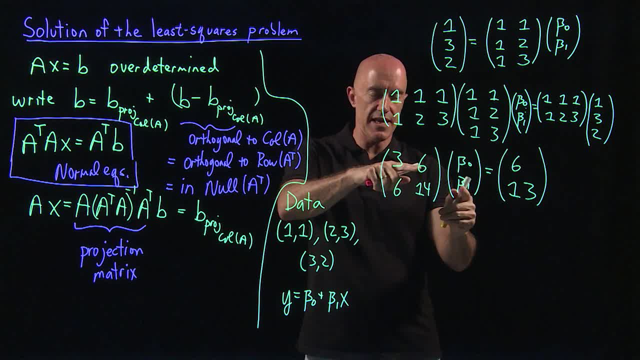 I think beta 0 is 1. And beta 1 is a half, So 3 plus 3 is 6. And 6 plus 7 is 13.. So beta 0, 1, 1 half will solve this right. 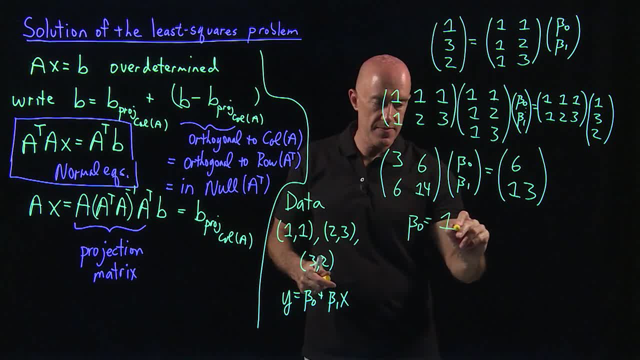 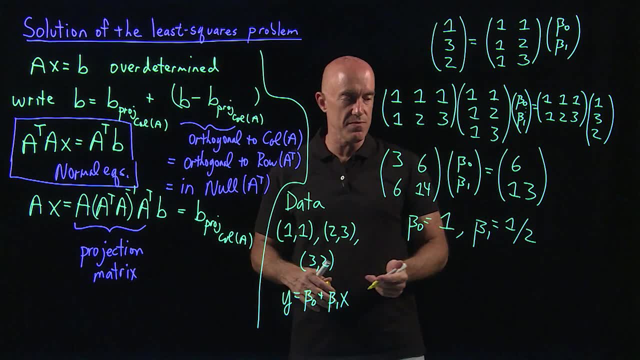 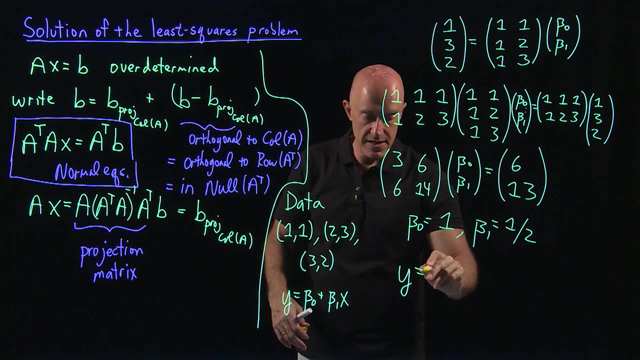 So this solution is: beta 0 equals 1.. And beta 1 equals 1 half. Very nice numbers, because I set up the problem so that the numbers are nice. So the best fit line then here is our Y. Y equals 1 plus 1 half X. 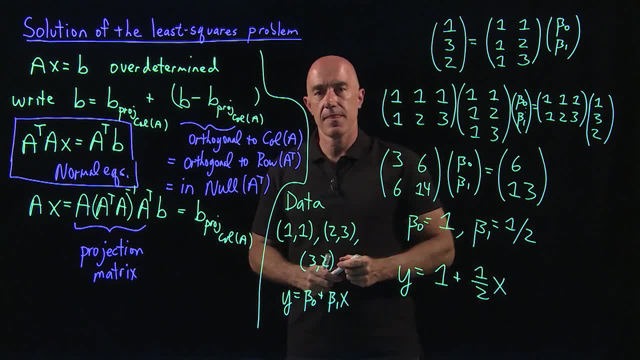 And that's the best fit line for these data points. Okay, If you look at the notes, you'll see the graph and get an idea of how good this is. So this is just a toy problem, one I can work on the board. 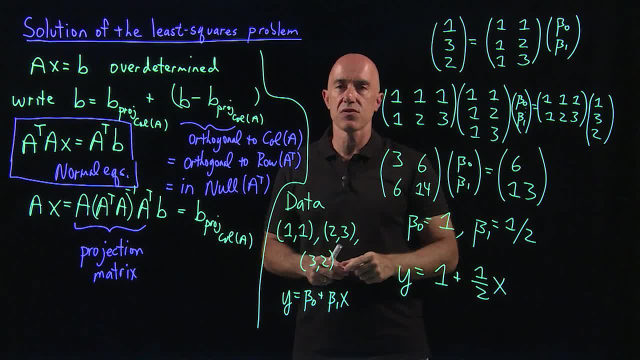 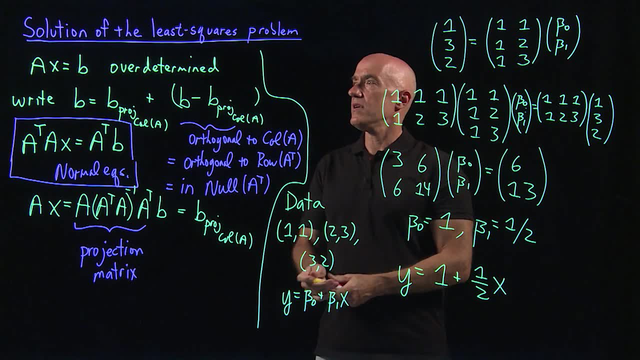 So we only have three data, But typically in a least squares fit, you have a large number of data that you're trying to fit a line through, So let me review. What I did in this video is to solve the least squares problem. 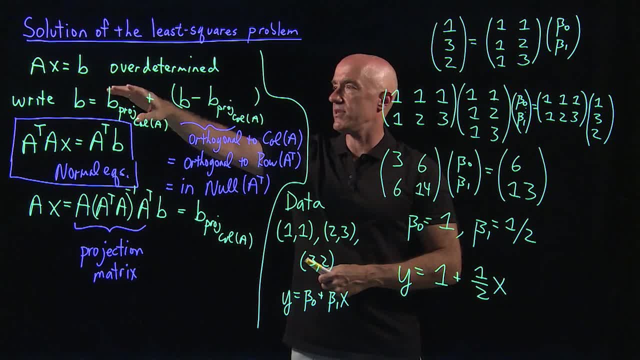 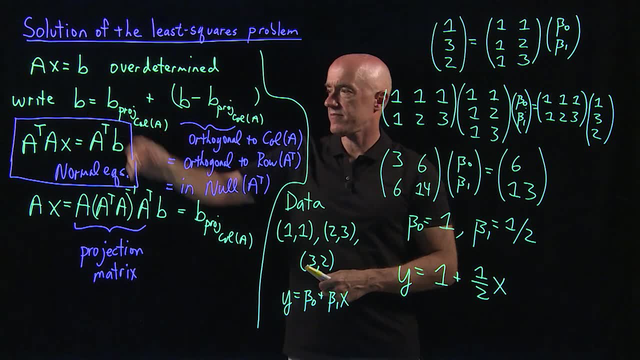 AX equals B is an overdetermined system of equations, So the idea then is to project B onto the column space of A. We can do that by multiplying both sides of the equation by A transpose on the left, And then we end up here then with what's called the non-transpose. 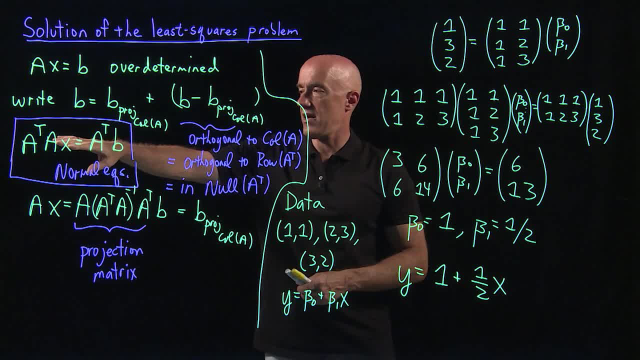 So we end up here, then, with what's called the non-transpose, And then we end up here with what's called the normal equations, which is a solvable system of equations. So A transpose, A then is a square matrix, invertible square matrix, and this equation-